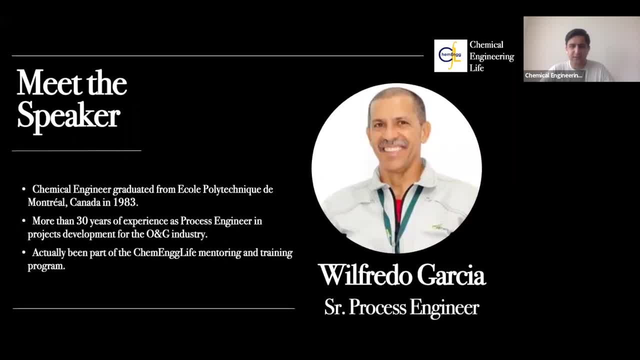 So first of all, welcome Mr Lopeto. He is a chemical engineer himself, with more than 30 years of experience as a process engineer in different projects for different oil and gas industry. He is originally an alumni of Ecole Polytechnique de Montreal, Canada, from 1983. 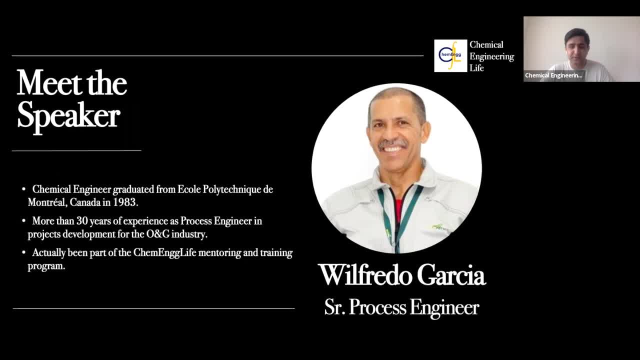 and he is a professor of chemical engineering at the University of Montreal. He is also a professor of chemical engineering at the University of Montreal, Canada. It's not the first time we have Mr Lopeto in chemical engineering life. He's actually one of our mentors currently. 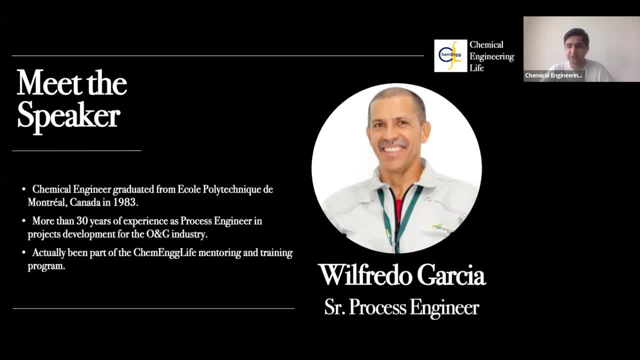 mentoring two different chemical engineering students and a major part of the training program- He and Mr Lopeto. apart from this, he also has different classes that he offers, so feel free to connect with him on LinkedIn and and also get get an opportunity to to become a. 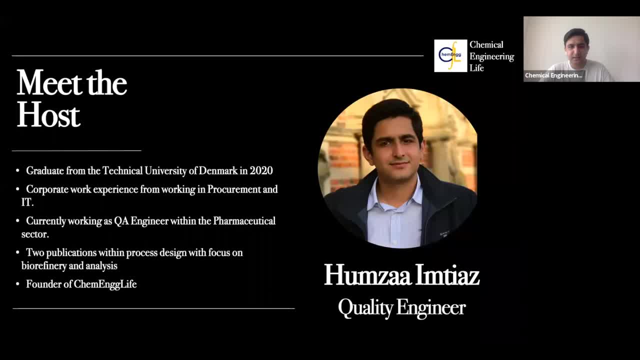 student in the classes that he gives A little bit about myself. well, I am. my name is Salman. I am a chemical engineer myself. I graduated from the Technical University of Denmark back in 2020.. Since then, I have been working as a quality engineer within a company called Leopharma, which 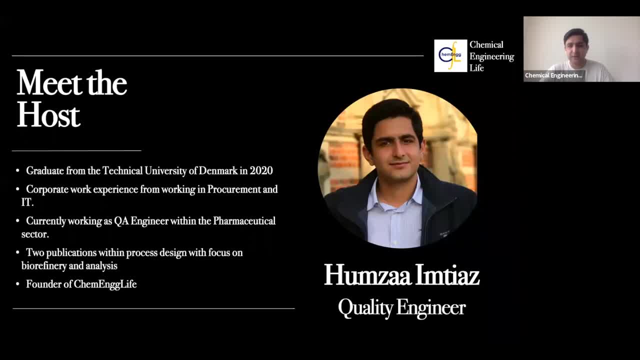 is a pharmaceutical and, within the pharmaceutical sector, My main focus during my master's has been on process design and process engineering, which led me to having two different publications within process design, which focus on sustainability, biorefinery and the process analysis, and I am the 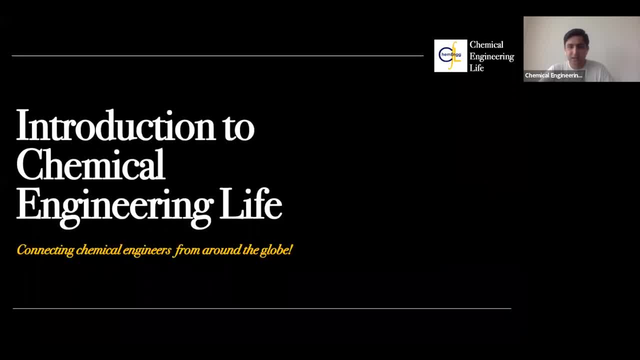 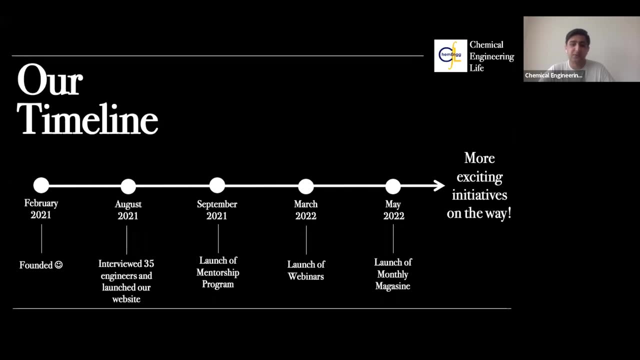 founder of chemical engineering life. Coming on to the organization chemical engineering life, well, the idea is to connect as many chemical engineers as we can from around the globe. A little bit about who we are: We founded the organization back in February 2021.. In the 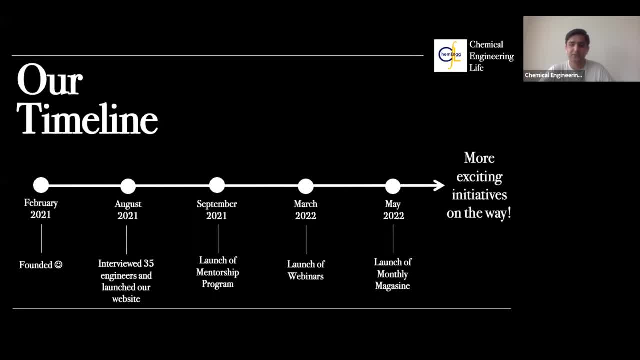 beginning, we started off by interviewing different chemical engineers. I reached out to different chemical engineers working in different fields, in different areas, different companies from different countries, asking them questions about chemical engineering. I also worked with a number of chemical engineers and I have been working with a number of chemical engineers and I have been working with a number of chemical engineers working in different fields, in different fields, in different areas. 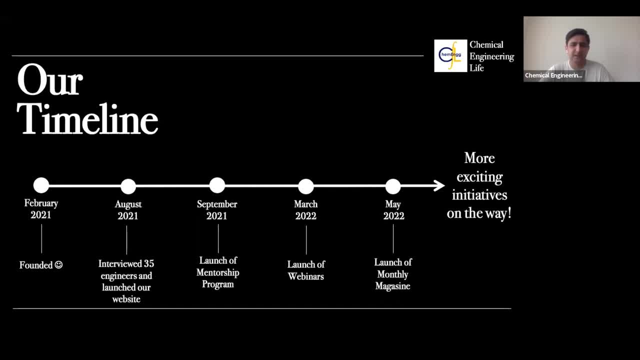 The idea was simply that we should be able to give an insight into the industrial life of chemical engineers for different graduates, for different students, So that they can get an idea about what to expect when they walk out the university gates. By August 2021, we had interviewed around 35. 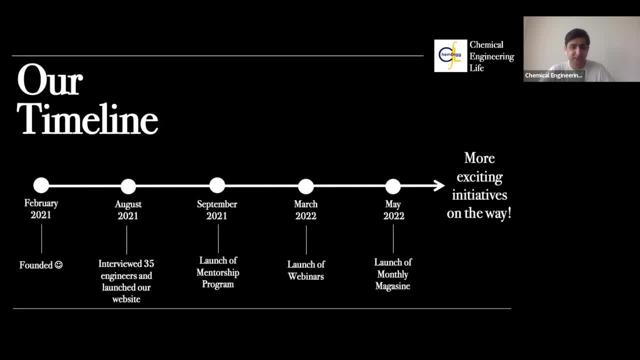 different chemical engineers. In the same month, we launched our website and all of the interviews can on our website, so feel free to visit the website and also look at the interviews. In September 2021, that is when we launched our chemical engineering mentorship program. 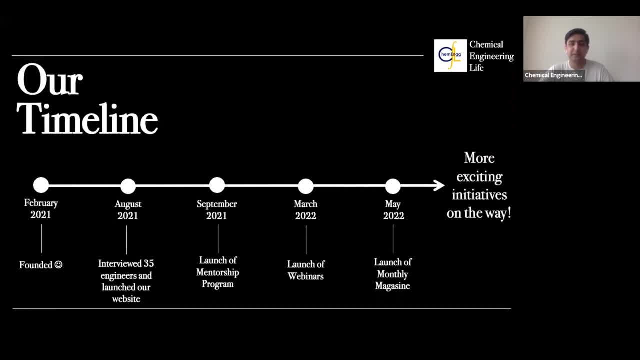 which is specifically built for chemical engineers. So all the mentors and mentees, they are chemical engineers from different countries And I will get more into that into the next slide. In March 2022, which is just last month, we launched our webinar. 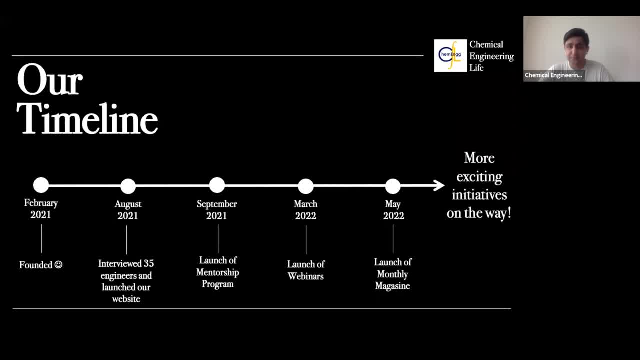 This is the fourth webinar that we are hosting with a guest speaker, and many more to come. So, once again, if you are interested in joining it, in signing up for other webinars, feel free to go to our website and stay updated on the upcoming webinars as well. 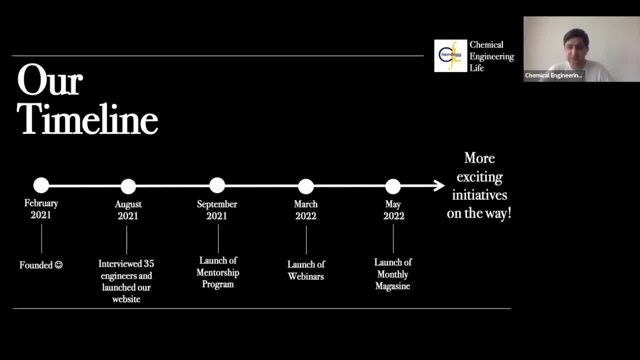 The next month we are launching our monthly chemical engineering magazine. It's a magazine discussing different topics within chemical engineering so people can stay updated on chemical engineering industry. So once again, go to our website and remember to subscribe so that you can get all the updates. 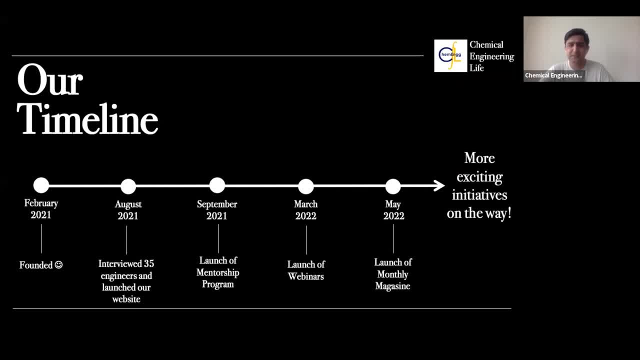 and get an online version at the end of every month. And this is just the beginning, As you like to see. there is a lot more on the horizon, So stay updated, And there are a lot more exciting initiatives on the way through which we aim to help. 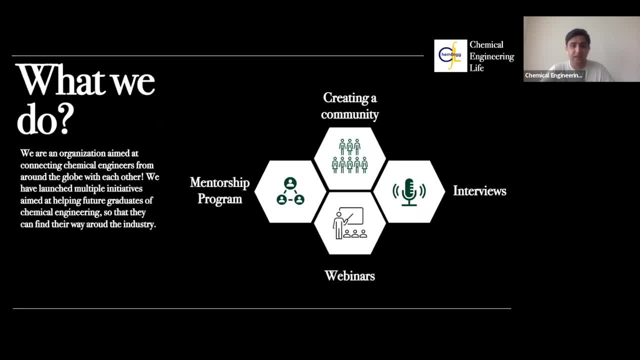 different chemical engineering students and graduates. So just a quick note on what we do. So, in reality, we are trying to create a community, a community where every single person you meet is a chemical engineer, a chemical engineering of different experience, of different sector. 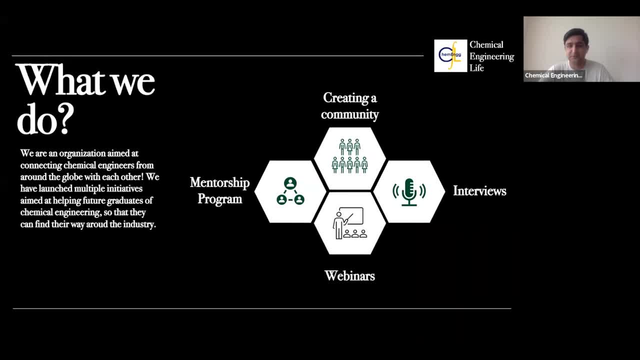 of you know, you think of it and we might have a person within that area, Within that community. we try to connect different chemical engineers with each other and try to benefit the students and the graduates by using the experience from industrial and experienced chemical engineers. 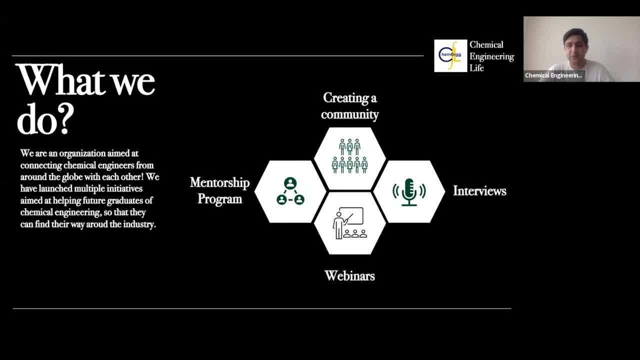 We do so by our mentorship program. the mentorship program where we connect different industrial engineers with different graduates, different master students, so that they can ask them any questions that they might have, Regarding anything from TV making to chemical engineering. we have these webinars. 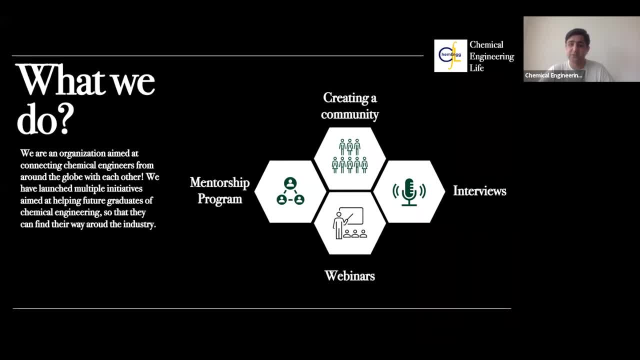 Every webinar we have a guest speaker who is an experienced chemical engineer working in the field or in the research area, so that they can come and give a lecture and many students and the attendees can get, can benefit from their content. And then, lastly, like I said, 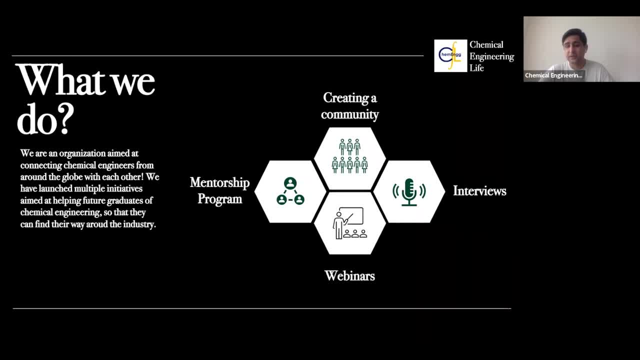 we have these interviews, the different chemical engineers. we do an interview every week. So once again, you can go in, you can make questions, send a question and we'll answer it. So if you have any questions, in and read their interviews and see what questions we ask them and what they answer. 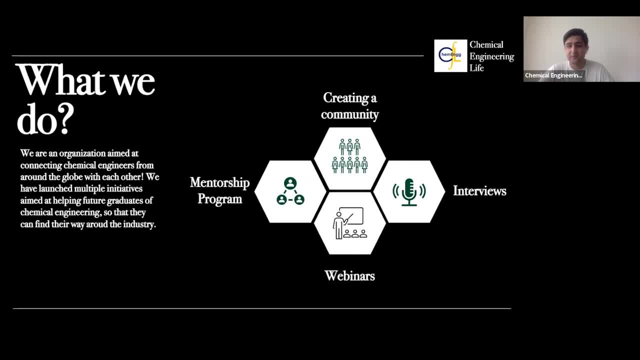 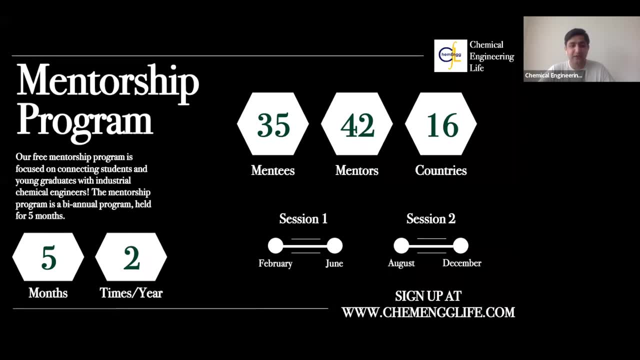 and you might get an answer to something that you might have been looking for. Coming back to our mentorship program, our mentorship program is a bi-annual program that is conducted for five months twice every year. The first session goes from February up. 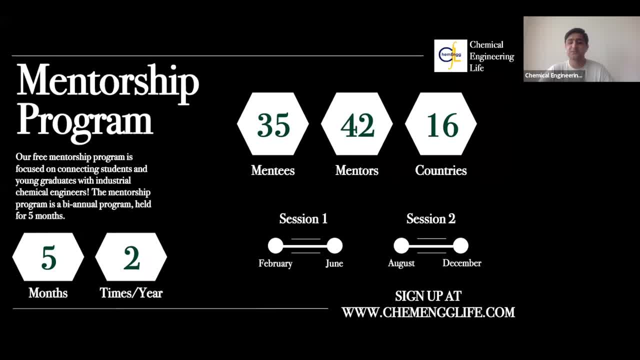 until June. The second session goes from August up until December. The session that we are running right now it is from February 2022 up until June 2022.. We currently have around 35 mentees and 42 mentors and they're all joining us from 16 different countries. We don't like to limit. 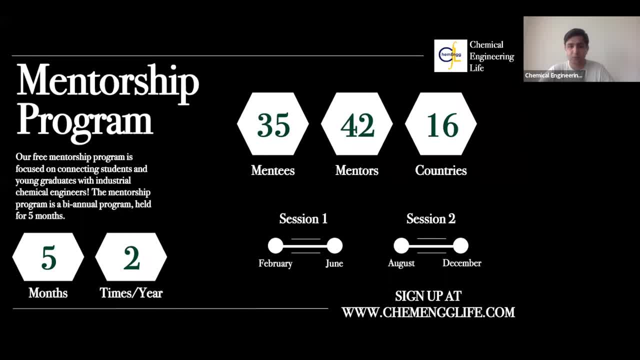 the program to one country or one university or just one, to simply one industry, such as oil and gas or pharmaceutical, but instead it is a very global program and it's a very open-ended program, so we don't dictate about what you can ask, What you can talk about, and I personally have a meeting with each and every mentee and a mentor. 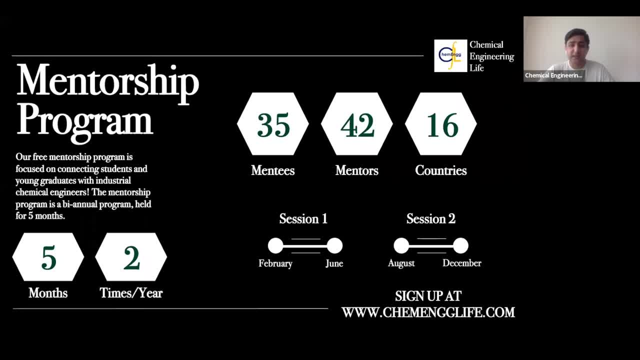 that signs up, so that we don't want anyone to be connected with someone on the merely that they are chemical engineers, but in fact every mentor and mentee are selected based on their own career goals and what they plan to do. So if you would like to work in the cement industry, we try our. 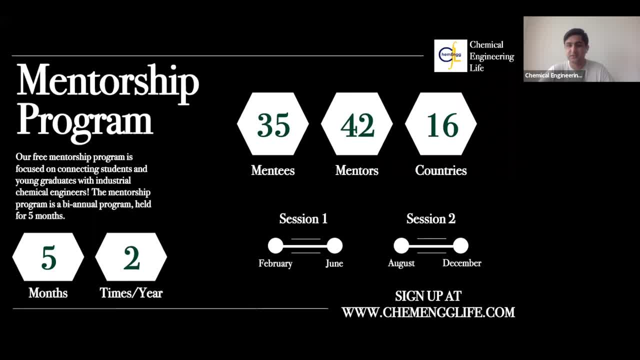 best to connect you with someone who is working in the cement industry so that you can ask them questions that might benefit you in your career. So do remember to go to our website, chemicalengineeringlifecom, and you can sign up for the mentorship program. It is no longer possible to sign up for the current session, since 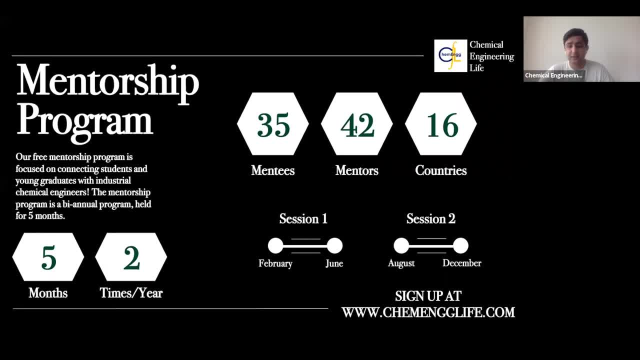 it is ending in two months, but we highly recommend that you sign up for the next session that we will be starting off in August, for which we already have started the interviewing phase. So if you sign up, you will be called in for a call within a week and we can have an interview to talk about. 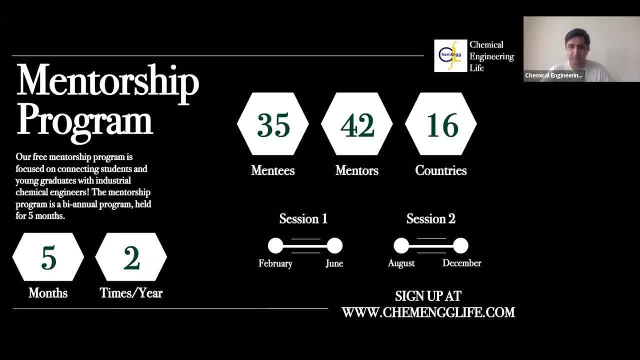 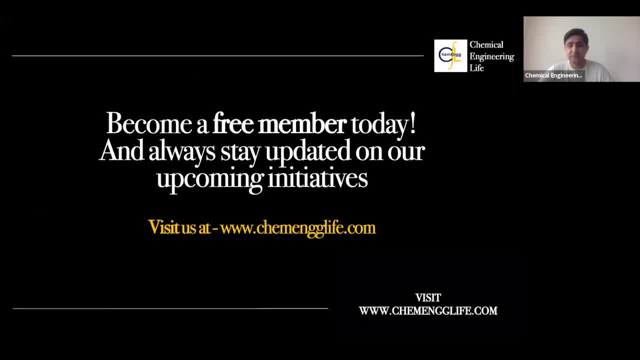 your career goals and what you plan to achieve out of the program. Lastly, on our website we have a free membership as well- The idea of what the free membership is- so that people can sign up and we can create a community so that people can connect within the 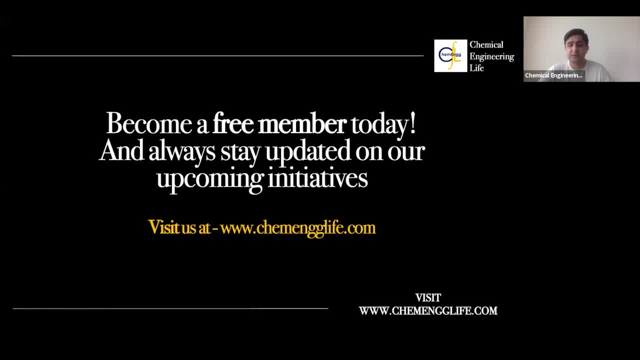 website with each other as well, out of the mentorship program and the webinar area. Like I said, it is a free membership, so you don't have to pay anything, but you do get a lot out of it. So go to our website and do sign up today. 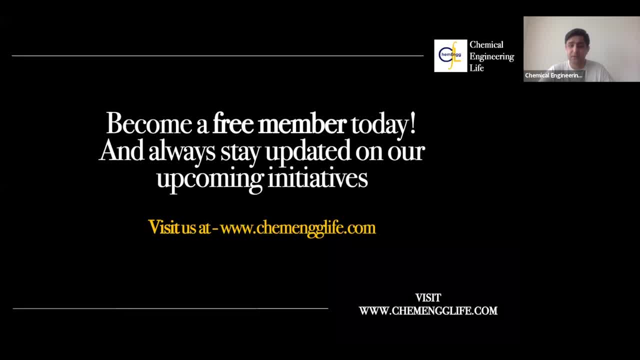 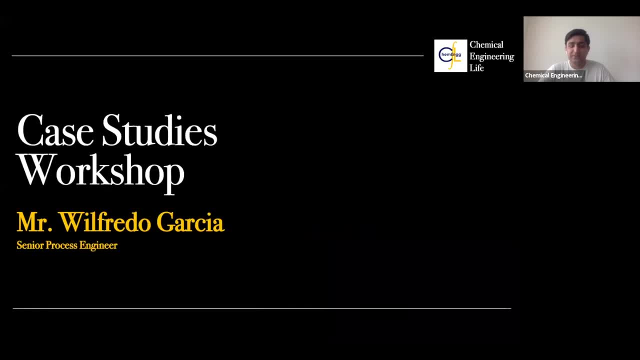 And if you are a member, you are the first one who gets to know when there's an upcoming webinar or if there is a new initiative. And that is all from my side about chemical engineering life. So, Mr Lopretto, you can take the take the lead now. 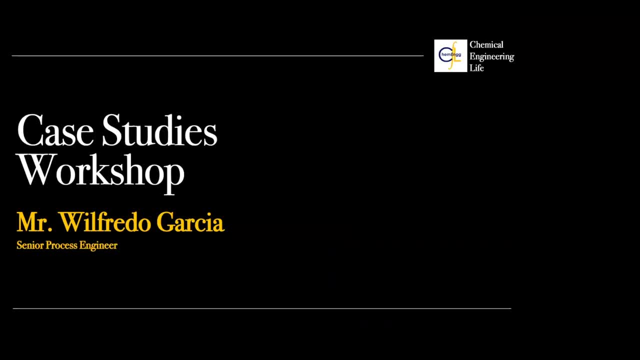 Okay, so good morning for me, good afternoon or good night for anyone else. Welcome to this workshop. It's called test studies because this is, let's say, a a situation that I have faced during my career on projects and in plant operations. 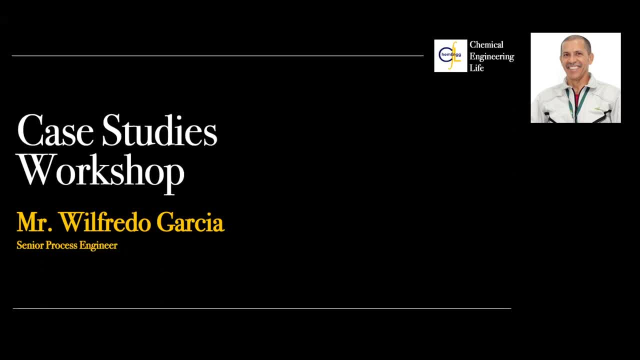 As an introduction, we, as a process engineer, one of our roles is to design safe and operable process plants. So during the design, we have to be aware of this because this is one of our role and the possibilities as process engineers. However, during the project development, 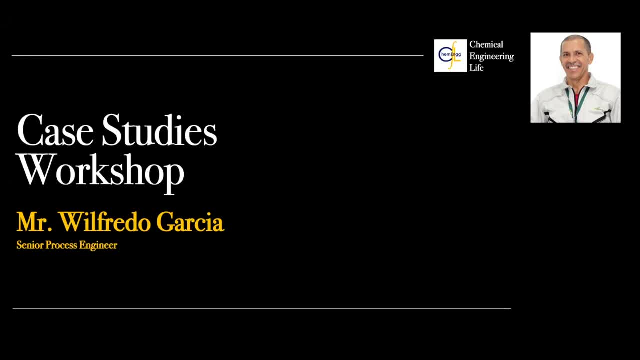 or during the plant operations. so there are situations that are less same. Most of the time are given because of pressure that the project management has from the client or from the plant owner to get this plant in operation very quick. So but us as process engineers, 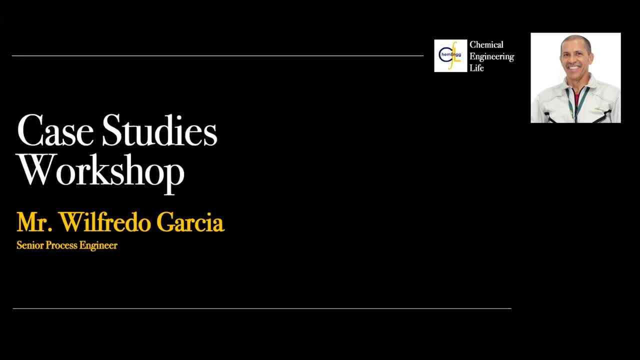 so we need to be aware of what is the kind of decision they are taking that are not affecting the safety of the plant- Okay, because the plant can be still in operation, however, so we need to be aware of the safety, For the safety is a very big concern. 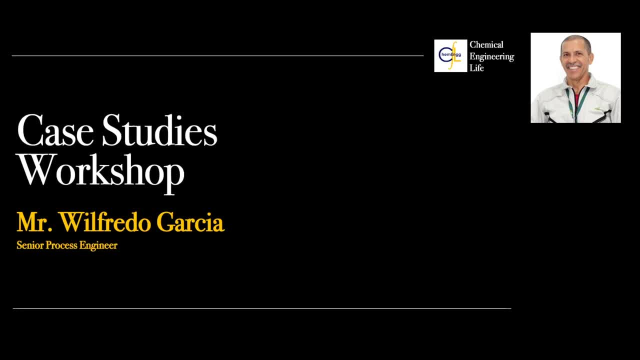 for the process plants And the safer the plant, so the happy that the owner or the client will be. So we need to be very careful. I see a lot of things in this because most of the time the people forget about safety. Because we want this project to be run. 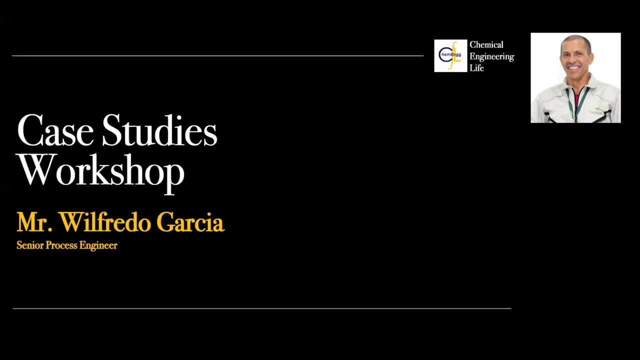 or to be ended in a very quick time. But most of the times the people forget about this topic, The process, safety management. it's a most important thing, Mostly not forgotten, just leaving, leave it away. So in this case, so can I scroll down Pulsa? 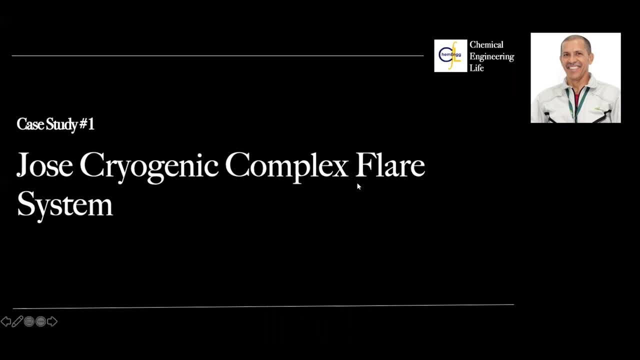 Sorry, here you go. I just selected. well, because of a matter of time, I just selected four cases that I have encountered during design or during plant operation. I have several. I have a lot of cases that I have faced. 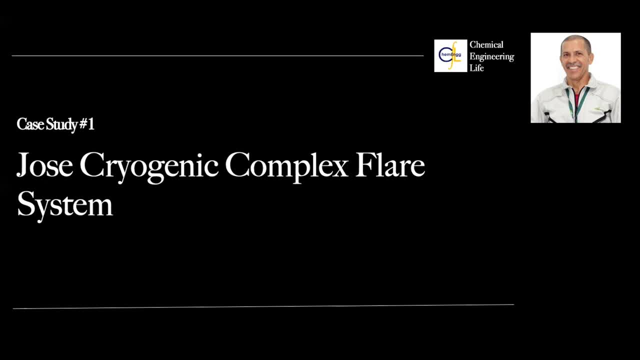 And then I have been. let's say, well, it's like fighting: Fighting with the project management to convince them to don't do this, or fighting with the plant operator to don't this way. However, most of the time so we are late. 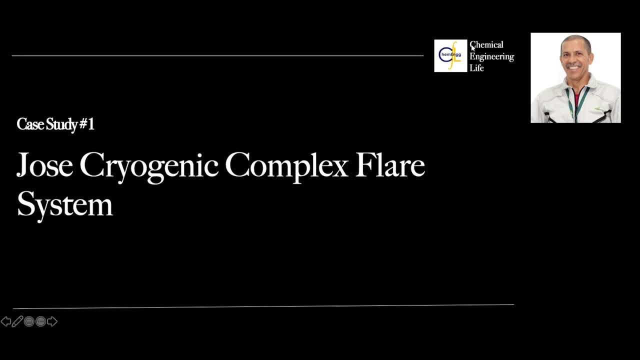 In this case, the case is already in place And then we have to take solutions, And then when they need solutions, they come to us As process engineer to give a quick solution to the problem they have faced. So the first case that is here is the Hose Cryogenic Complex. 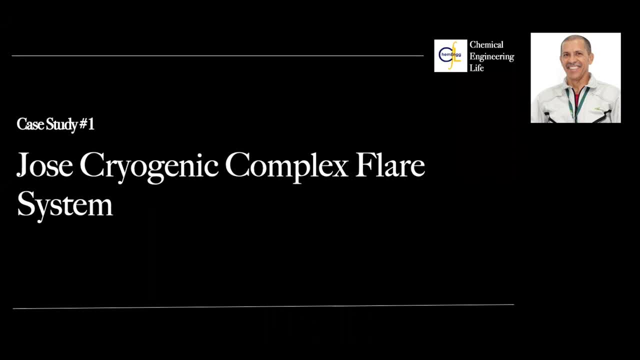 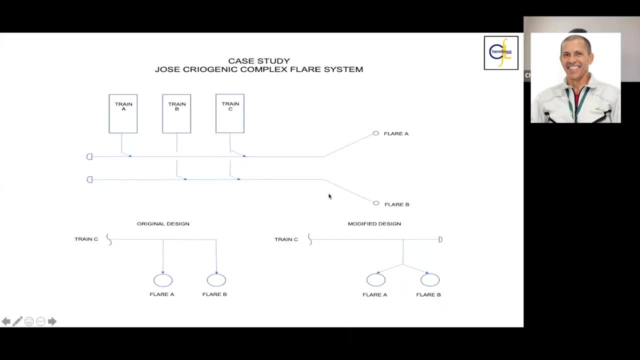 It's a complex, that is, so I cannot scroll down Pulsa Please next. next, So the Hose Cryogenic Complex. so it's a process plant, that is, it has been built to process NGL, So natural gas liquid. 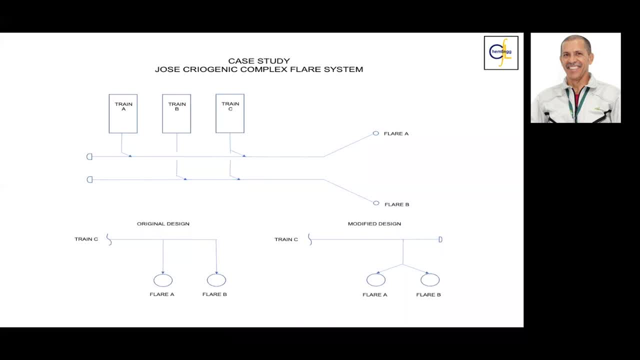 The natural gas liquid is being generated or an auto gas processing plant. off string of this, It's called a Santa Barbara gas processing plant. They take the natural gas, they dehydrate, they take all the treatment for the process plant And they extract the NGL with a maximum 2% of ethane. 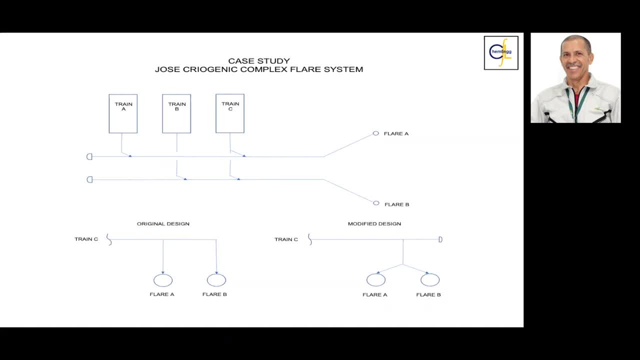 that is being fed to this Hose Cryogenic Complex that I was working in. this project, This train that you see here- train A, B and C- So the train A and B. they were built to process 35 million, not 35,000, barrels per day. 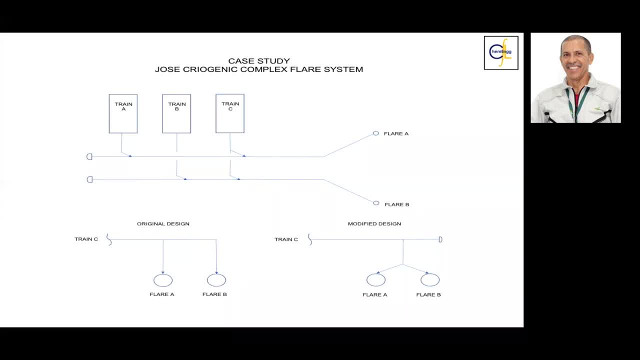 And then the first time we get into this project, so what? to upgrade this train A and B from 35 to 50, to process from 35 to 50,000 barrels per day? Okay, And then in this complex, so they receive the NGL. with a maximum 2% of ethane. this NGL is reprocessing the NGL with a maximum 2% of ethane. So this plant has several distillation columns to recover propane, N-butane, isobutane, N-pentane and gasoline. 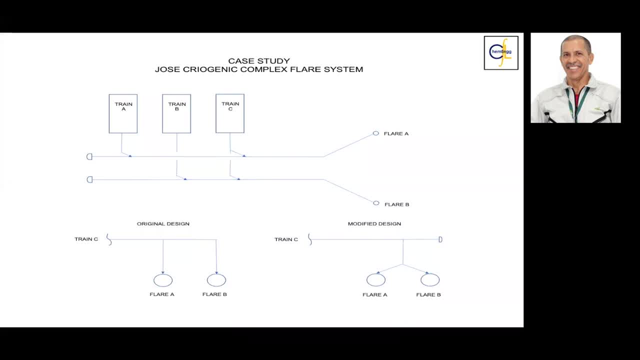 So this is the main product I'm interested to process is propane, normal and isobutane. Those are the main products they commercialize in this train, So the first project I worked with them was to upgrade the train A and the train B from 35 to 50,000 barrels per day. 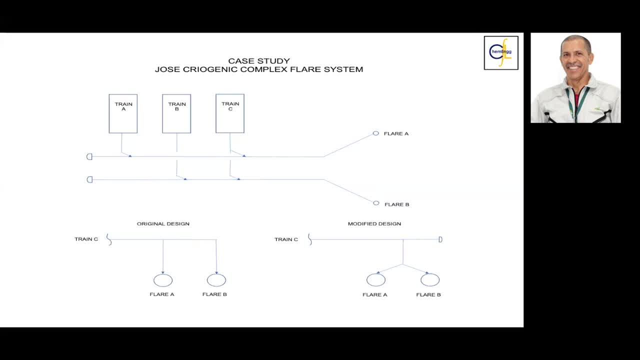 Okay, However, so this is the part of gas processing, but we have to see what happened point of view process safety management, because any of this train has its own flare system. So there is a knockout drum here that I didn't show you. 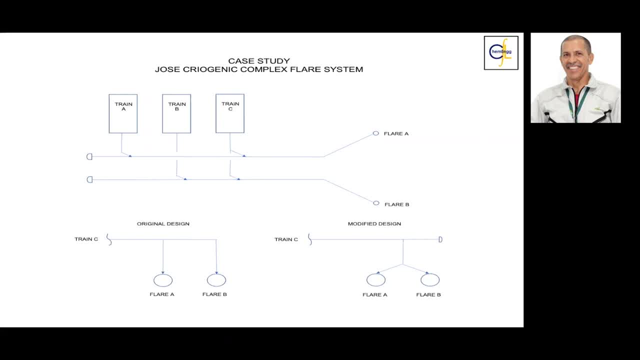 because it's not necessary for this case study. I just showed the flare header and the flare itself in that sketch. So any train has dedicated flare. flare for train A, flare for train B. After we finished and completed the upgraded project from 35 to 50,000 barrels per day. we have to go to the next project, And this is the first project, This is the second project, So the last project is for 20,000 barrels per day, at 250,000 barrels per day, the demand on propane and isobutane. 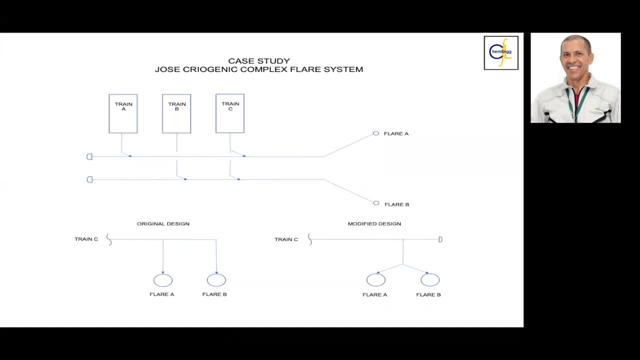 was still increasing And they introduced another processing train in Santa Barbara field that allow for this plant to include another 50,000 barrels a day train, A processing train that it was called train c okay. however, the train c now has its own flare system. 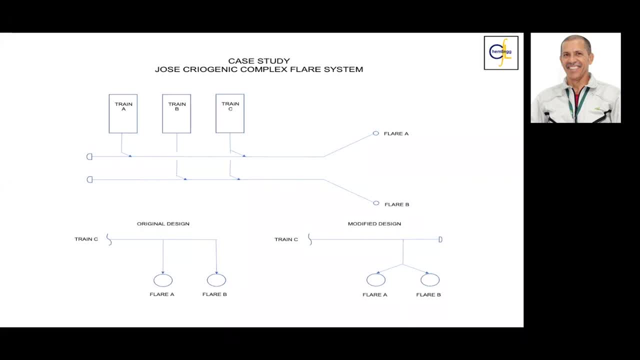 correct. and when we run the study of capacity of the flare a and b, so we notice that the train c cannot be incorporated in one flare but we incorporate it in a couple. so we split the relief header in two in the four to, let's say to when the gases to both flares. okay, 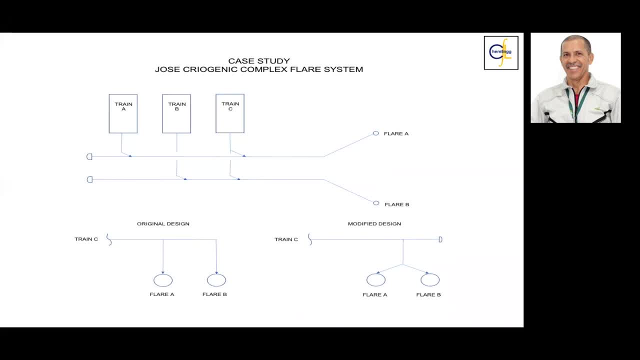 but the problem was not there. the problem was no capacity. this flare a and b during when we study the several scenarios on the maximum flow rate at the three trains at the same time. so the flares still has have got capacity to process these cases. however, the problem in here 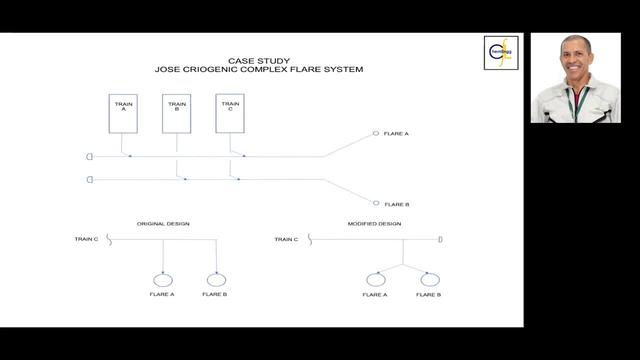 was the connection. how do we interconnect this train c into these two flare? so at the beginning of the project, so we didn't focus on how to do it. we just say what we want to do with this soup, with this flat header from the c, and then the connection has been done in that way. okay, we have. 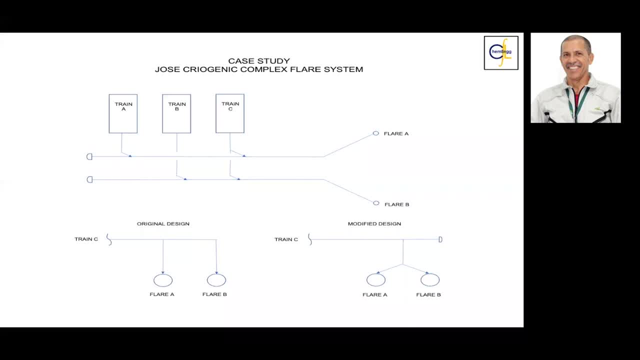 this header. that is there and it's feeding. very simple. we split in flare a and flare b. this was okay, it has been built, the piping group has done this job, etc. however, when we were doing the commissioning, so prior to start of the plan, so we test everything and then, when we try to test, how was the behavior of this? 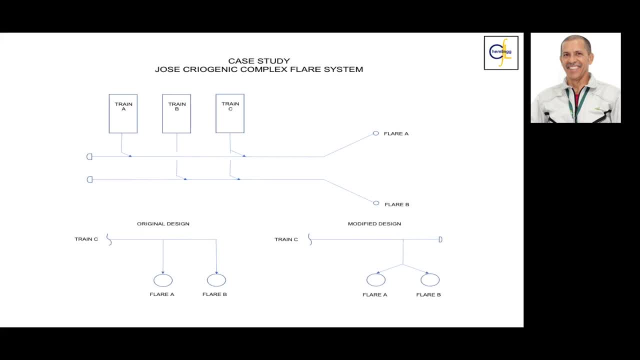 connection there. so, uh, we introduced one, uh, a potential venting that's similar to the flare capacity. and then what happened when this um system went in operation, okay, for test the venting, and then all the flow go to the flare b. so all the flow go that way, okay. and then what happened that in that, in that place, 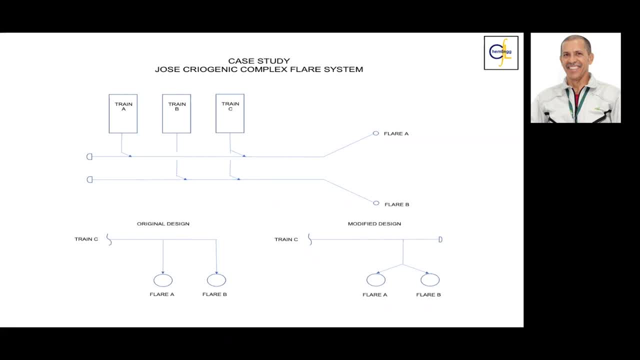 so, uh, that effect, uh, generate a vacuum in that section. and then what happened? that the, the flame of the flare a was woof, was thin. so we noticed that we were in the plan testing this, and then suddenly we didn't see the flame of the flare a, because here the flow rate was flowing that way and generate a vacuum. 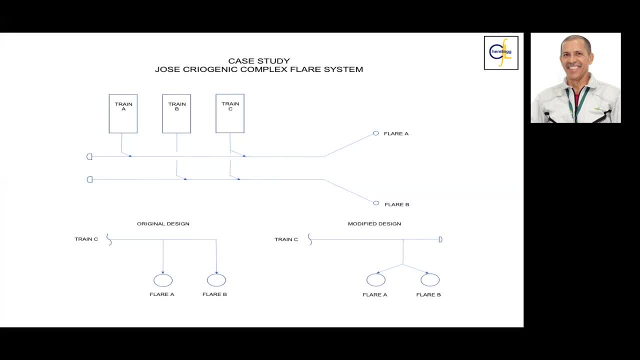 okay, this was a problem of connection. and then we needed to do something very quick, because we were in commission commissioning that plan, and then we have to run a very quick study, so well, let's say dynamic hydraulic study, to find a solution for this connection, to avoid, so, to get a proper 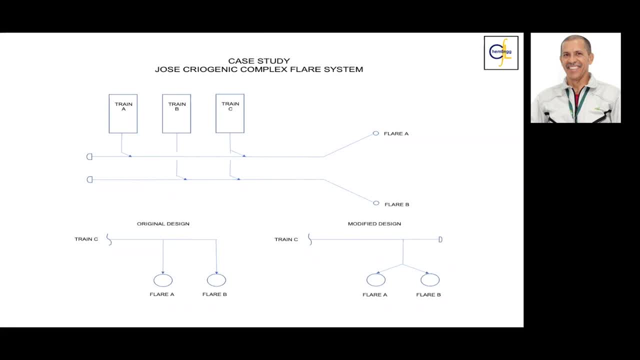 distribution of the flow from coming from this connection to avoid, so, to get a proper distribution of the flow from coming from that flat head. and then we run some study and then we got a- uh, the conclusion that the best, well, it was not a 50: 50 distribution, that we got there with that. 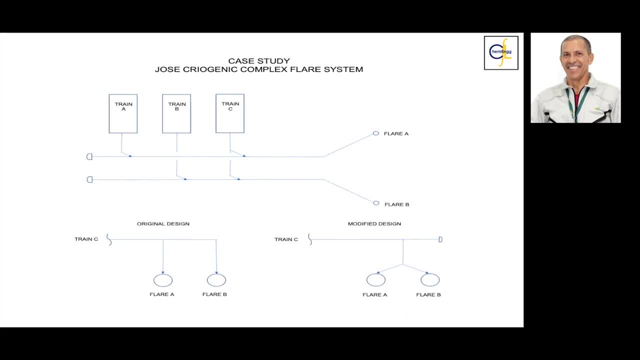 arrangement, but this was the best solution that we could give to that- uh, let's say distribution, and to avoid that relation. it that a vacuum effect in that connection? and then the the connection was to include one, so to extend the header and to include something to stop the flow rate coming from there. okay, because all 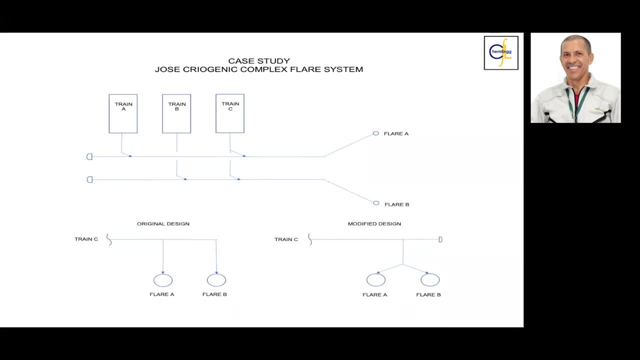 of you remember the newton law: that is, something is moving in one direction. it will not stop. it will try to continue moving in the, in the in that direction. and this happened as well when we are dealing with fluid flow. this, this in: we introduce something to stop. 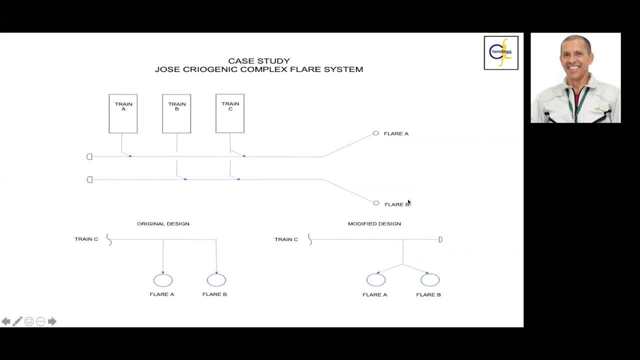 to try to stop the flow in that direction and then to, let's say, to obligate the flow to go that way and then to split in something like- uh, i don't remember the angle we have there something like 60 degrees or 120. i don't remember what was the algorithm on this, but this is the best. 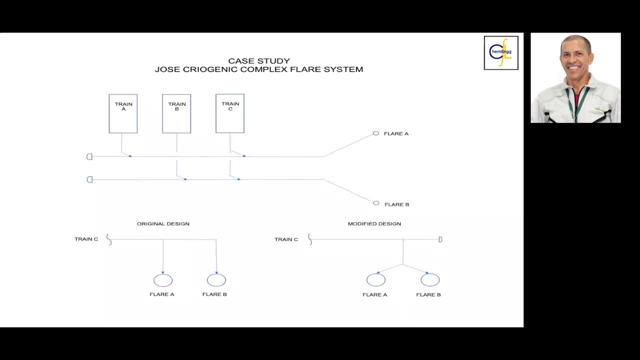 arrangement we need to this flow distribution. and then, when we tested the game, so the flare a maintained its flame. that was the purpose of this, um, of this study. okay, the distribution, as i say, was not 50: 50, as we wanted, however, so the solution was: 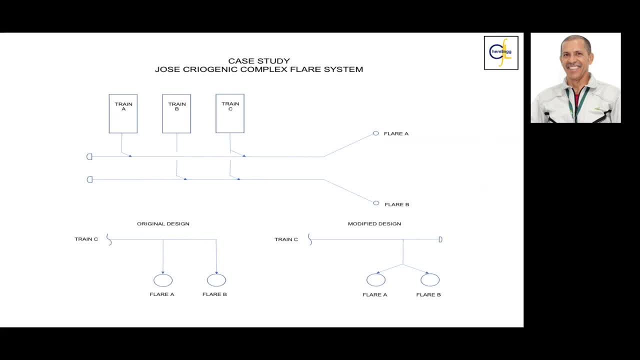 something by uh 52, 48, something like that, okay, but the purpose of this, to introduce this change, was to get a best, a better flow distribution of the uh, the flow okay, and to avoid this. and then this is one thing that i am, i am, i bring this case. 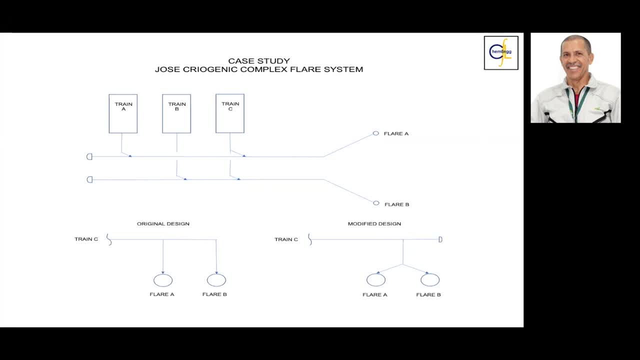 this case study to this webinar because we as a process engineer, so we have to take care of this very early. don't wait until the uh commissioning phase or during the the um, the, this, the detailed design phase to run this kind of studies in case that we have it in our project. this is the purpose of this: to present this case. 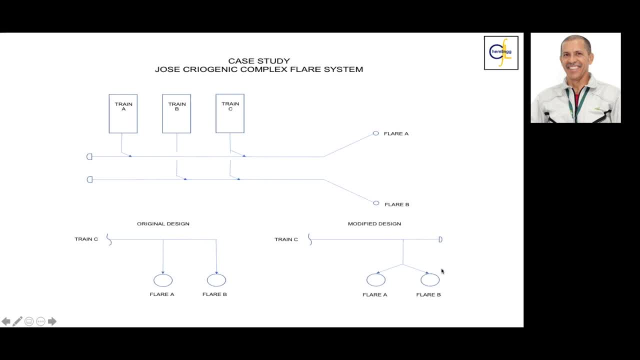 study. so don't don't wait until it is too late, as we say, as i say always in during the project and during the life, when the water is at your, at your legs, so say so: we are floating. don't wait until the water is there to say that we are floating okay. so take action very early, in the stage of the 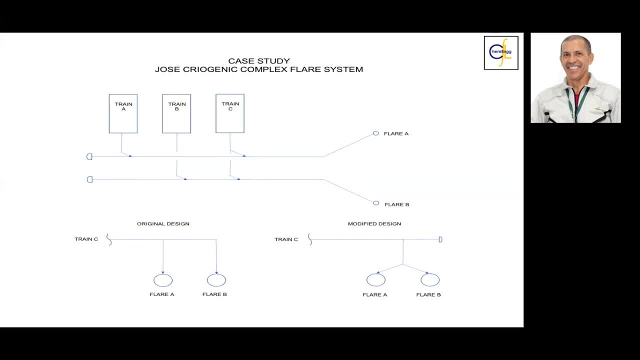 project to avoid this, because we have, we have to rework, we have to do a rework in that project and then we have to do it very quick because we were, let's say, handing over the plant to the owner and then we would so during commission that we, we see this, we didn't. so nobody, nobody see. 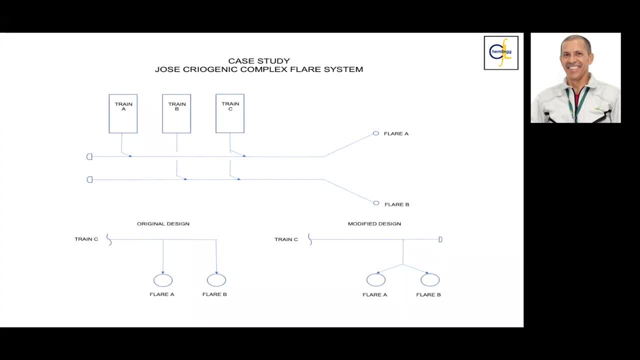 that this arrangement will cause that problem during the design. and then, and don't forget something, uh, we, as a process engineer, we deal with a pnid, so in the pnid we show this. however, is the piping designer that make the design. and then, when the piping designer is making the design, 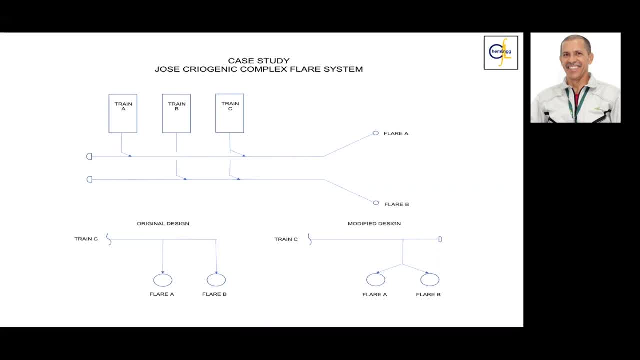 it's very important for us to get participation in that particular design, because this is something that is, uh, relating to process safety management. and then if we go into the 3d model, if we participate in the 3d model review, it is very important for us as a 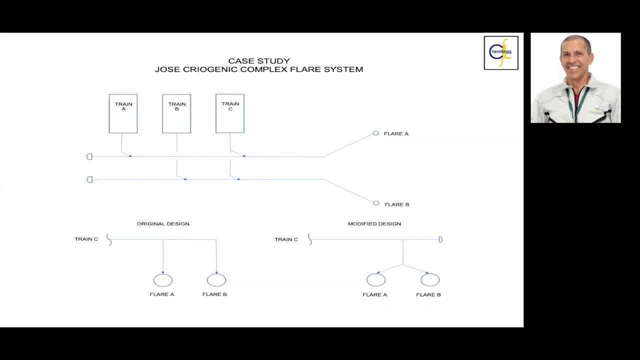 process engineer to participate in those models, even if you are saying to don't participate. please talk to your project management, to the project manager, because most of the time the pipers piping group make the best arrangement for them and then if we see there, so we have additional costs because you have additional material. 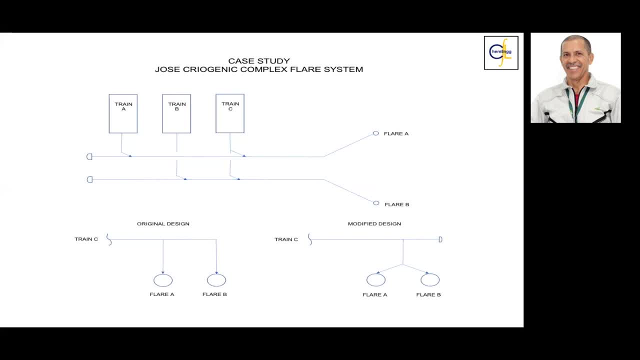 to be introduced in that arrangement, rather to use that arrangement, and then so it's uh, remember that in in the um, in projects, here we have a triangle. a triangle, all the projects is managed at the end of the project. So you have costs, you have time. 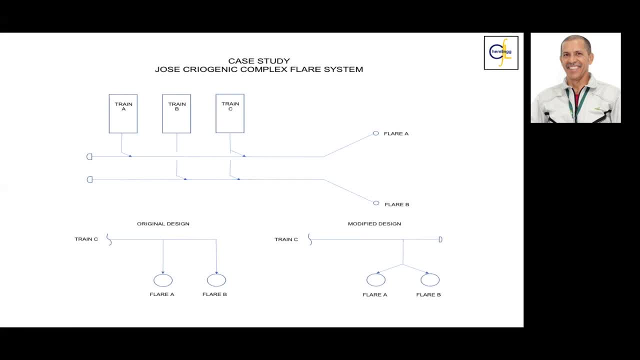 or schedule, and you have quality at the other extreme, and then these three variables are in equilibrium. anything you do, so this triangle will move. somebody will pay the price. okay, so, uh, most of the time we are under pressure during projects, but remember, we, as a process engineer, we have to do. 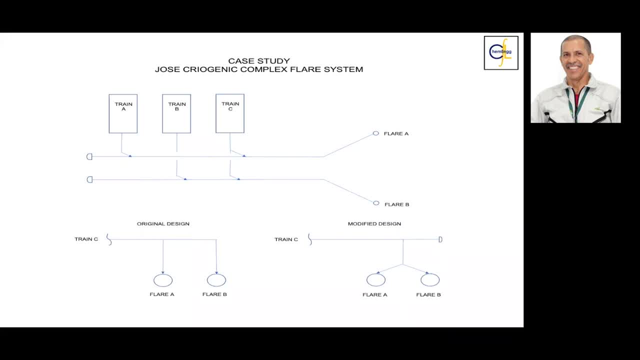 thing in a good mood. so, and then, everything related to safety. please, please, put the eye on safety. don't just say that i have a process simulation, that everything is fine, that i have got the number, my item material balance is okay, because this is okay. this is the normal way to do project. 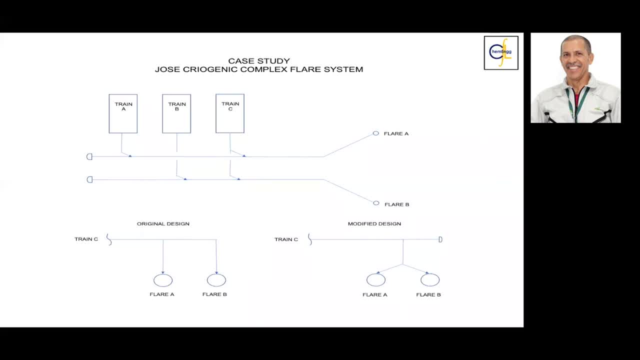 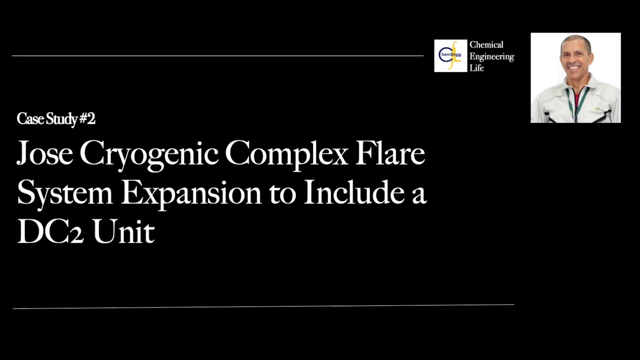 however, when we ought to do this, what was the safety management? so please open your eyes, okay, yeah, let's move to the second one, that is, the other case study that is in the same cardiogenic complex, but in this case they wanted to operate this plant with the ngl, with ethane and the ngl. 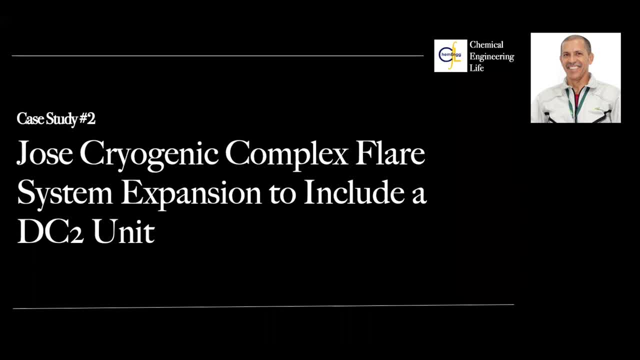 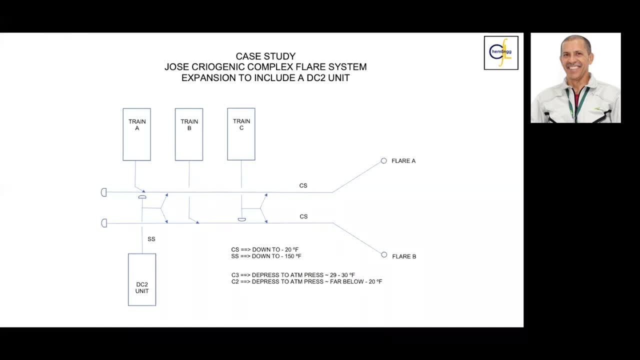 without it. that is the case before. so please, who's the next one? and then the next one. we have the same case situation. so already we have these three trains in operation with the solution in there for the interconnection, and they wanted to introduce one, the ethanizer unit. so they say to bring ngl with. 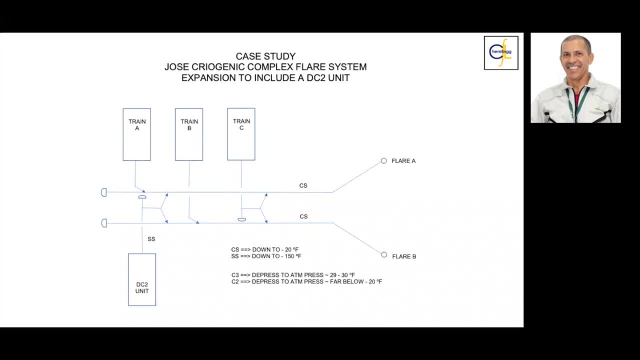 more ethane and then to process the ethane in that complex as well. the point of view project it was very good. so we have area to introduce all the plants, we have area for tankage, we have area for refrigerator, we have area for the refrigeration. 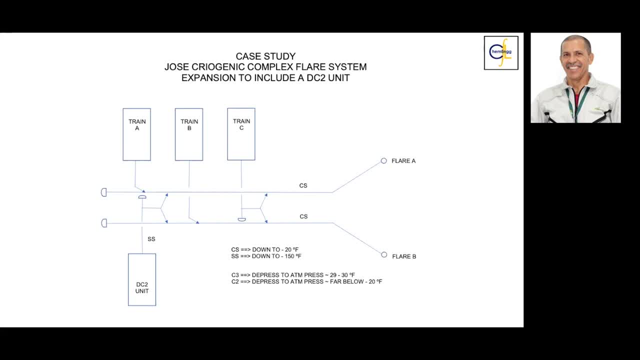 plant, etc. point of view process, everything was fine. however, point of view safety management, it was a problem because the owner of the plant- they wanted to use the same flare system that is already installed, and this is logic because it's a matter of cost. so we already have flaring facilities in in the process plan, so i don't have to invest in a new. 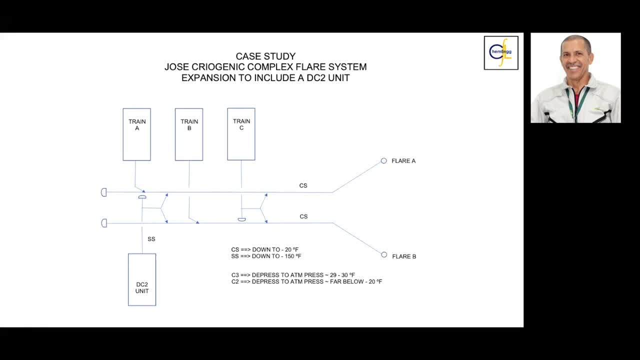 flat. so, if you see the situation from this point of view, so it was very easy because it's a matter of course, however, you were compliant, or safety, and the reason is very easy when, well, if we see the material construction, the material construction from the uh, this, the, the ethanizer unit, is pretty 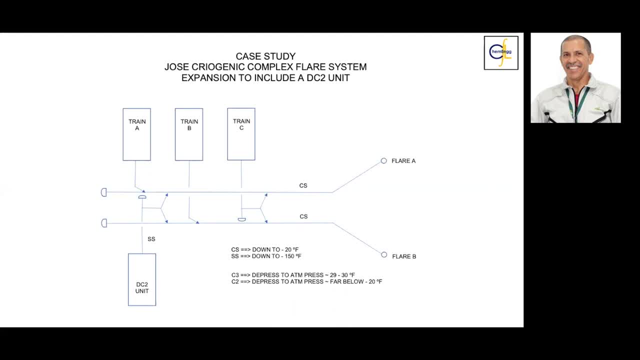 good. it's mostly stainless steel and the existing flare and the city and the material of construction of these three trains is carbon steel, mainly carbon steel, because we don't- we don't face lower temperature. the carbon steel point of view, one of your resistance and stress, is very good down to. 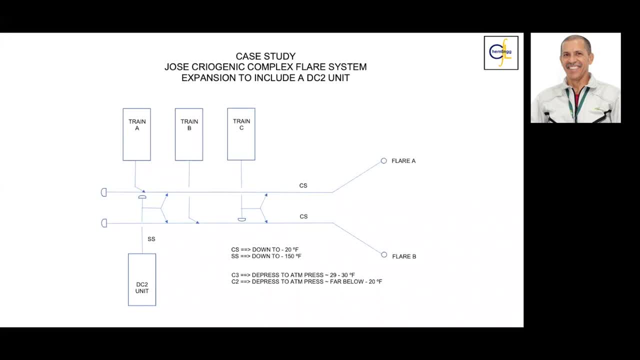 minus 20 degrees. finally, and the stainless steel is very good too, and another load: up to 50 and lower temperature, talking about cryogenic conditions. however, when we, when we start to look at this- so in this time we learned the lesson from the previous exercise- we say no, we don't, we will. 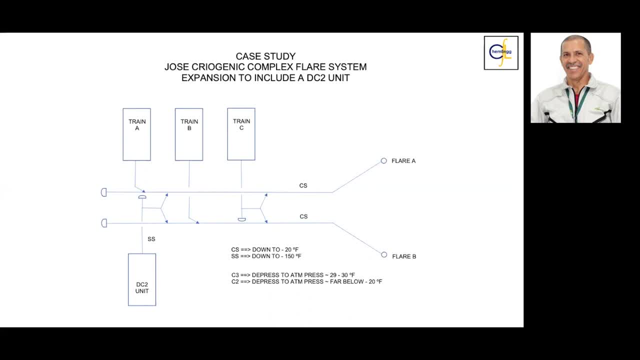 not see this at the latest phase of the project? let's take it early. what happened? we run exercises of the pressuring, the um, the, the compounds that we have there, okay, and then in the for these three trains mainly, we have the lighter product that you have in there is propane. when you depressurize the propane to 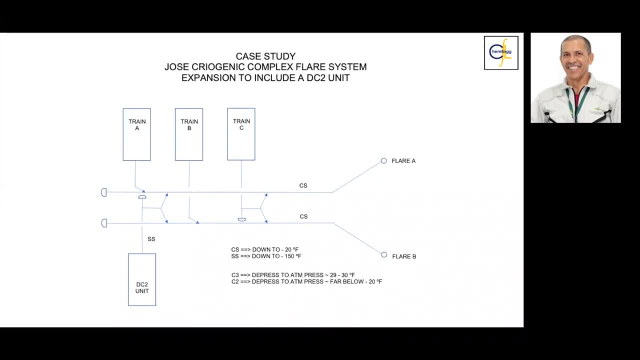 atmospheric pressure, because this and the flare is some close to atmospheric pressure operation. so we got not 29 to 30 degrees, fine, but we're going to exercise. however, when we depressure, the lighter thing here, this heating, so the resulting temperature is far below minus 20.. 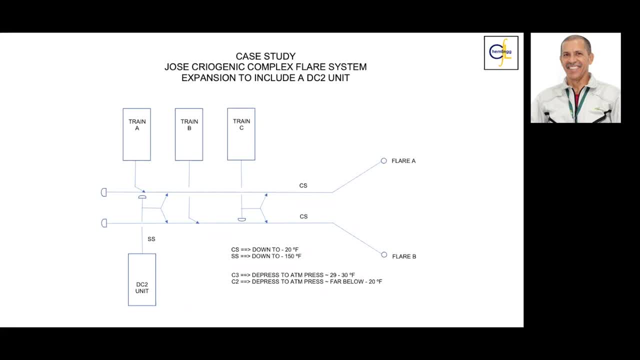 so with this very cold temperature. so this carbon steel material will fail on the real mechanical. so material selection, so the carbon steel will will not withstand one depressuring or one or one flare release or one vent release from the, the eternizer plant, and this creates a problem, a big problem and a big discussion. 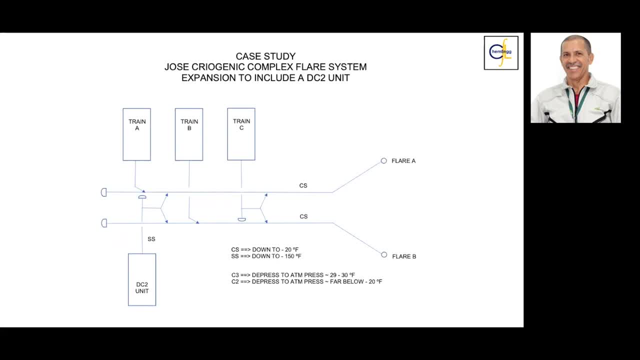 so the project management was angry with us. the, the owner of the plan, also was angry with us. say what, but what is the problem? so you want to run a safe plan, as we, as a process engineer, will do so. you have to install a dedicated stainless steel flat system for your heating plant. you won't. 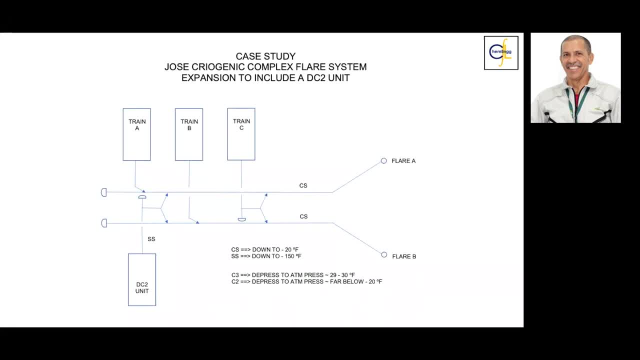 want anything at the euthanasia unit in your complex, you need to invest in a new flat. but now it is. it's costing money. that this money, they didn't estimate it when they propose, when they get this proposal. okay, so this was so they they needed to introduce a new budget. 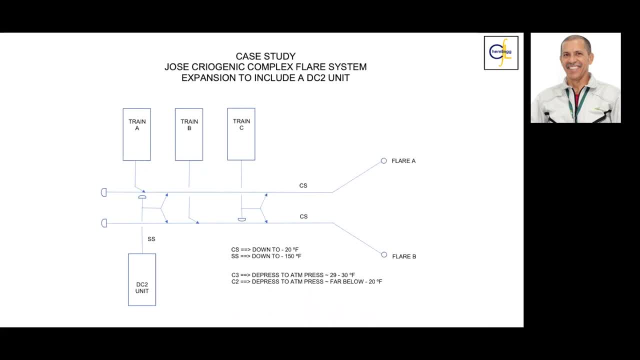 into the management of the owner of the plant so that to be approved, prior to introduce them, to include a stainless steel, a flare system. and then we needed to convince everyone, starting by a process manager, because they wanted to run this uh project very fast, because it was very ease, very easy because the plan was already you know, say, the size of the area. 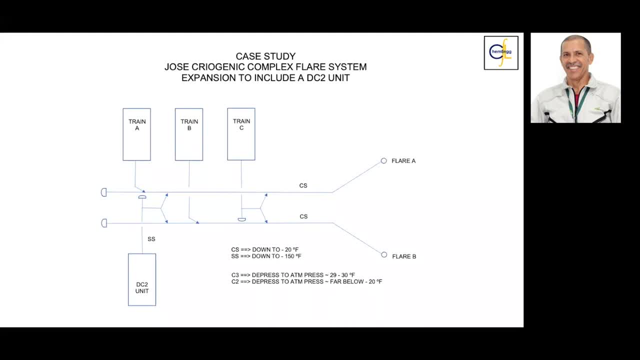 already. you know be what they have the nåd textured, these narrowed, and they are even equipment was already there because they pick one train from the Santa Barbara extraction plant, the same size, they put it in here with the same capacity, 50 million barrels per day. okay, 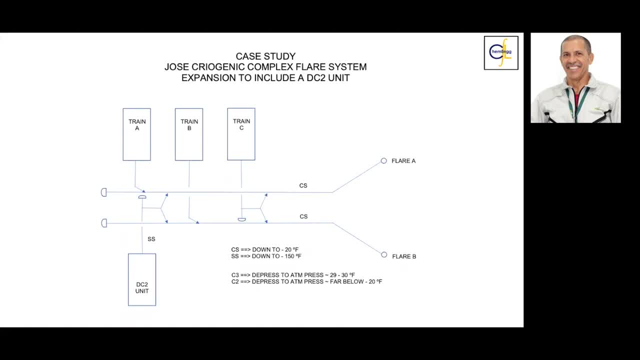 The same capacity, no problem with this. But however, we have this constraint point of view, process safety management, And then at that time everybody insisted that we have to do that. And then we as a processing engineer we say okay, and then even the owner of the plant 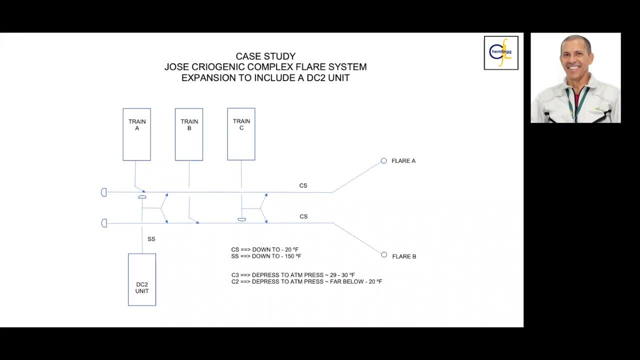 they say, they tell us: no, this plant will never be depressurized. And we say what? That this plant will never be depressurized at the level of pressure. this plant needs operation. Okay, if you want this plant to don't be depressurized? 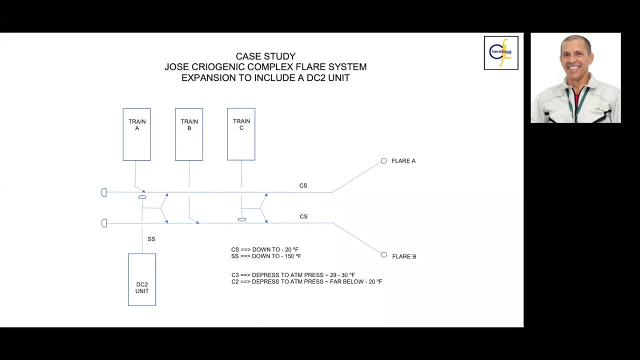 please, let's write one letter, So you submit a letter to us that this plant, the depressuring of this plant, will be in your hands, And then the failure of the carbon steel will never happen. Please write this to us, for us, as a process engineer. 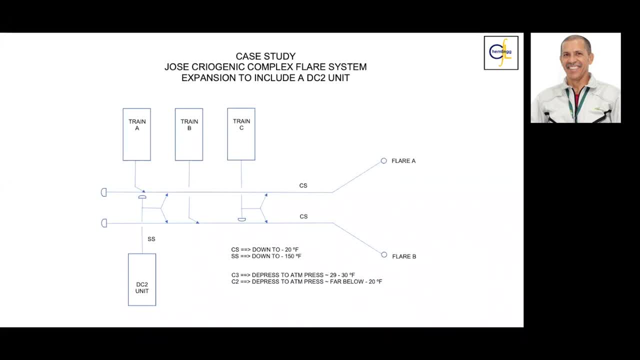 to be free of warranty or responsibility of this, because we didn't want to be responsible for something that we know that in the future will happen, because sometimes this plant will need to be depressurized. So, whatever the situation is, you can not say no, I will not do it. 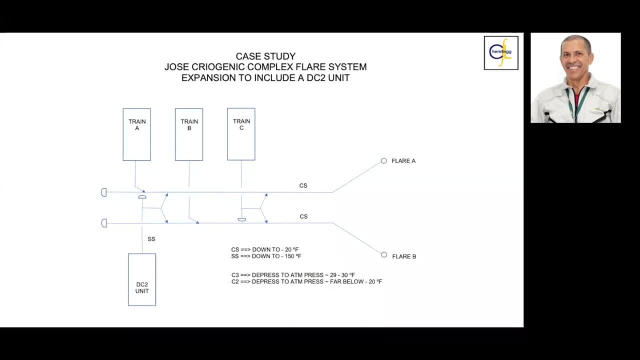 No, no, no, no, this will happen. Okay, fortunately this project didn't go further, And then this unit so has not been installed in that plant. Fortunately for that plant. so this project was put down, But otherwise so there will be a big 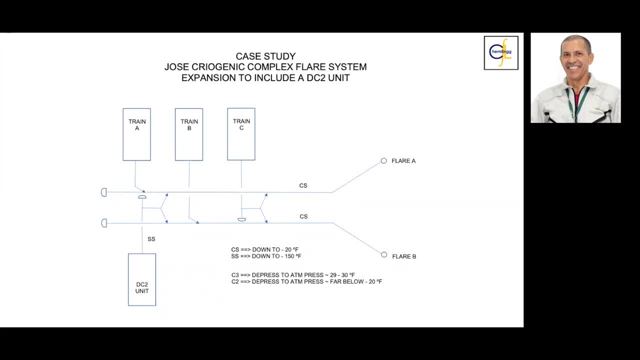 big safety problem. They will introduce into that a complex, But this is as I say. so sometimes people don't understand. People is thinking about money, money, money, money, and they forget that in any project, even in your life as well. 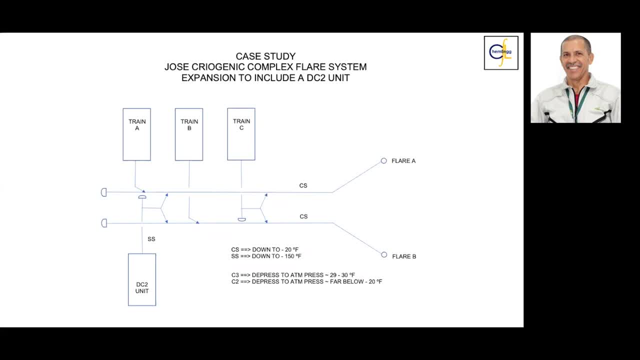 So you have another two variable, that is, quality and scale. So you try to earn money, So you need to invest. it will take more time or it will take quality, And they need the safety is in gaming here. And then, when we are talking about safety, 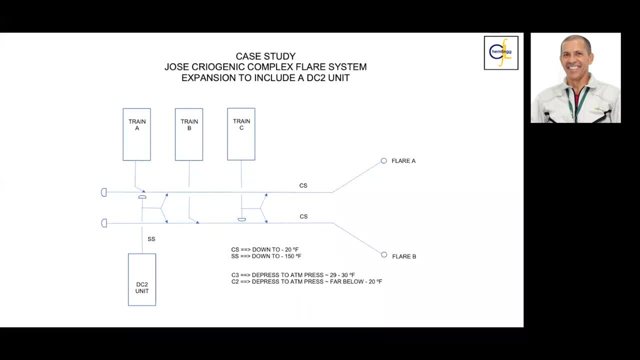 forget about the rest of the variable, my friend, because it can lead to a very, very, very big problem. Can you imagine that this material failed for any reason? Yeah, the carbon steel crack and you have a leak of this light product in that plant. 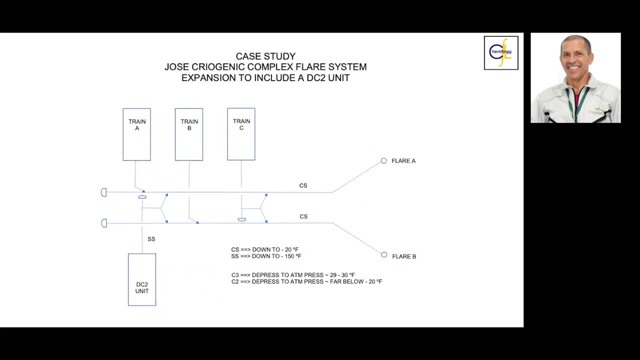 So you cannot imagine the emergency or the problem that we have in this. So this is another lesson we learned in this project: that this dealing with material selection. Okay, so if any of you are working with cryogenic systems, for example, LNG production, 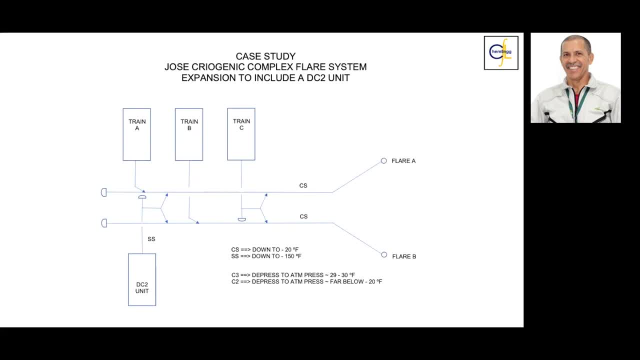 please be aware about the material selection, Because I have another case study for one LNG plant, but I see that I will have no time to present it in this way in this today. Maybe in another webinar we will talk about that or there, Or if we speak on LinkedIn or in another. 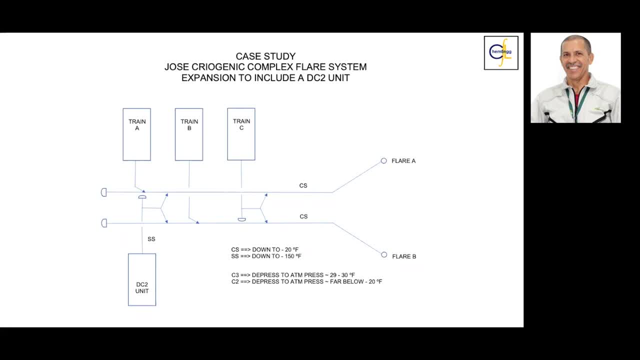 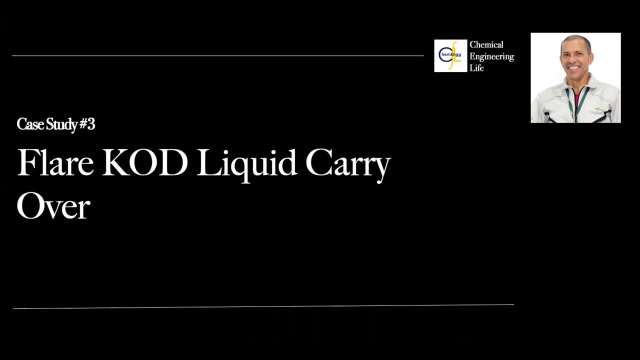 communication I will let you know what happened with that plant And in other cases that are not only regarding design but plant in operation. Can we move to the next one? The next one is what is called FLIR knockout drum liquid correction. In fact, this is what happened. 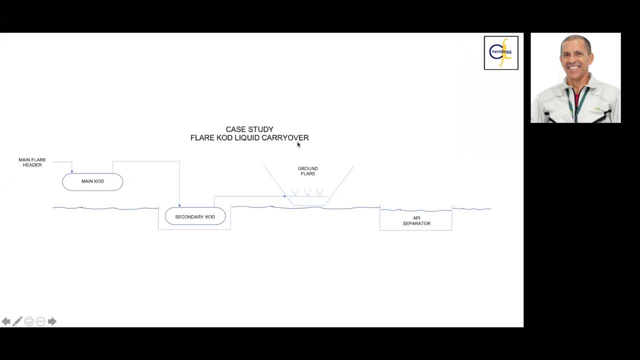 So please do this sketch to explain what is going on there. So we have been called to run a study for the FLIR systems because there were several systems for the El Palito refinery in Venezuela. Okay, they say that they have a big fire in the air. 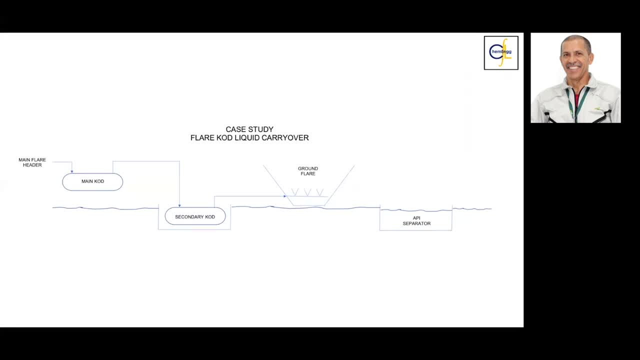 And it is the same thing. They have a big fire in the air, in the air, in the air. So they have a huge fire in the air in the air, And the reason for that is because they are not using this system. They are using the other systems, the API separator, because they have a liquid carry over from the main account. 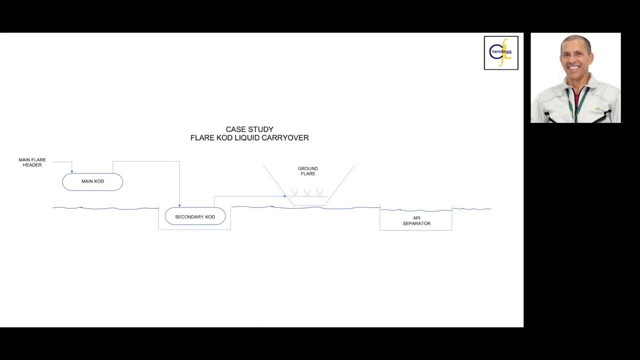 This main account is linked to the FLIR header from the process plant in the refinery, Okay, But they have maybe five or six relief systems going to the ground as well, But these are several and other plants. for example, they have an aromatic plant that they they wanted to segregate from that stream. 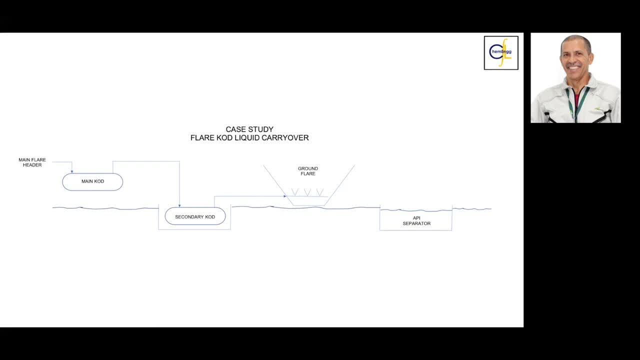 they have an oxygenated plants that they want to segregate as well, and then they they have several a um flesh system going into the same ground player. so they say the ground flight has a very, very, very high capacity. however, the problem was with this system in particular, because they have one emergency in the refinery plants and then 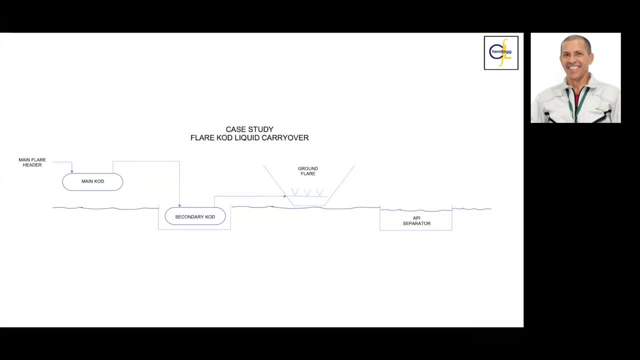 when this um peak, a gas flow rate went into that knockout drum. and then this secondary knockout drone is very small compared to this, so they have, let's say, a liquid there burning. okay, they have, they don't have gas, they have liquid. so they have the bullets burning in there, and then the wind direction, which is that way, and then all this um. 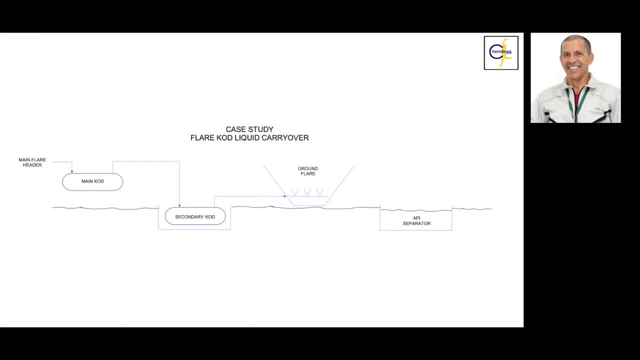 firing balls, they drop into the api separator and they have a big fire. in that case, this is the reason they say they wanted for us to run a study to to check the capacity of the fresh system, and then it's one study we did so we pick information from any, every relief. 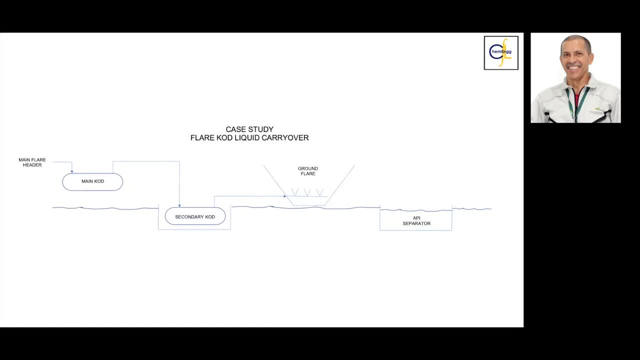 or heavy pressure safety valve and pressure relief in plant. we made the analysis for any of this system. for the header, we noticed that it's not headed requires to be interconnected, as we did that before for the a and b? um, because the capacity was. The problem was back pressure. for the pressure safety valve that was very high, they were selected, for example, conventional valve. and for the back safety, for the back pressure that required to be changed to a pilot valve, but this was not the case. we didn't want to do this. so we need to interconnect some flare header to, let's say, to minimize the back pressure. for another case, 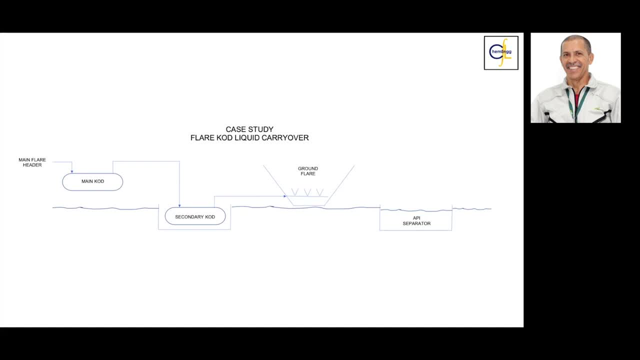 But in this case we check the capacity of this knockout drum and then we say okay, according to the normal operation of the plant. and then what we've got, the information we've got from field regarding the liquids coming into this flare and then the liquids that are, let's say, condensing during the flare. 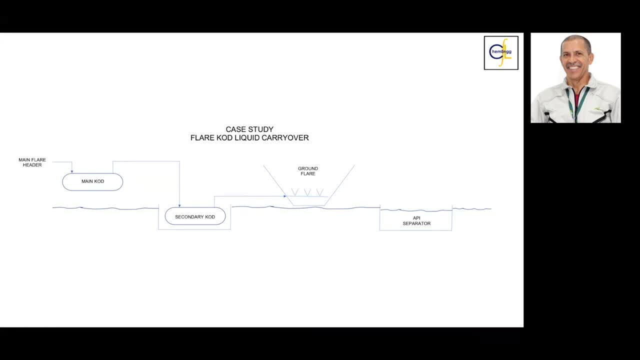 release. so this main knockout drum was okay and then this is the conclusion we have. so we have no problem with the flare knockout drum. so it has enough capacity to manage the liquid that is expected to be here and then to manage with the maximum flow rate that is expected to be here, because remember that in the main knockout drum normally you have no liquid. 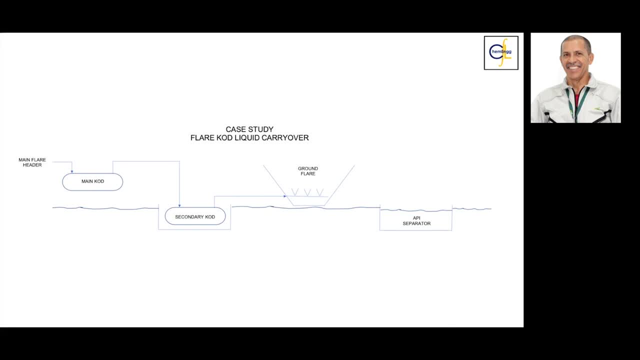 Okay, when we have a release from a pressure safety valve, this stream is mostly gas, so we have few liquids. and then just to size this KOD, so we specify one volume of liquid there and then you have, you install here a pump that starts and stops, so it's an on-off pump when it reaches a maximum level. 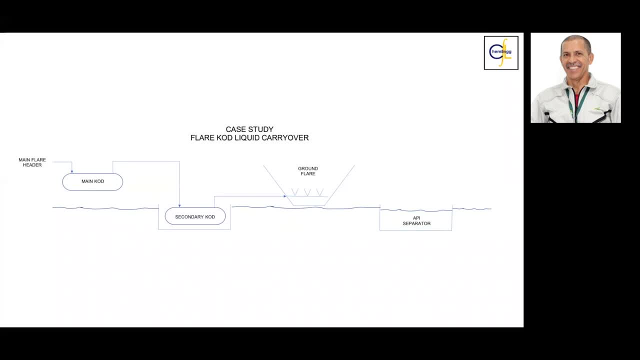 start. when it reaches a minimum level, stop and then normally these pumps here have maybe 50 or 100 gallon per minute capacity, so we are not talking about big pumps in this and the operation is on-off because you don't expect liquid to come, so a huge quantity of liquid to come with these streams during the release. 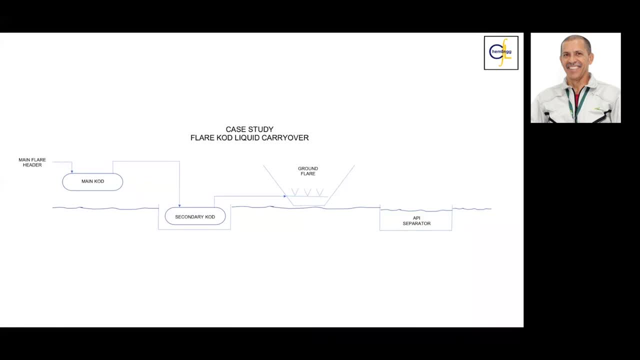 However, when we were there in the field looking for information- so we have got- or some operators, what was the real cause? So this is another lesson that we have to learn from all the studies: we have to look for the root cause of the problem, not to deal with the consequence, because we already know the consequence was that you have liquid in there. 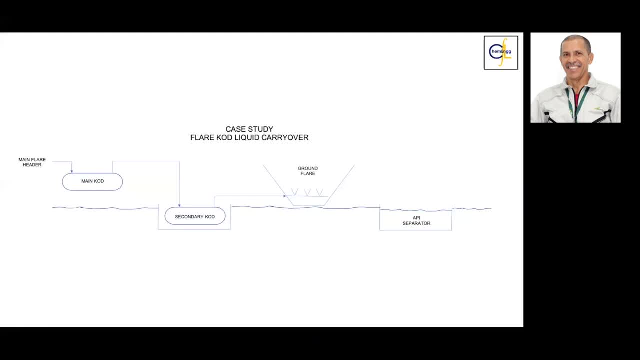 a burning liquid that cause a fire. But, however, what was the root cause of this? And the root cause is one of the operator tell us that they have to say to blow down the alkylation plant in the refinery and they don't have any tank. 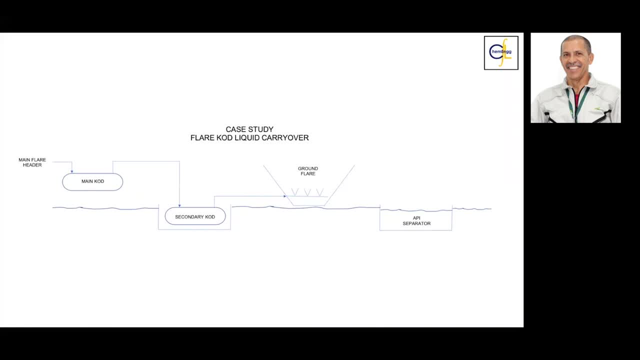 to allocate that volume. And then somebody came with a big idea, because this main knockout drone is a very huge pressure vessel, Looks like a horizontal tank. So you see, the side will drop back because it's quite big. And somebody say, okay, as the fact that the flare 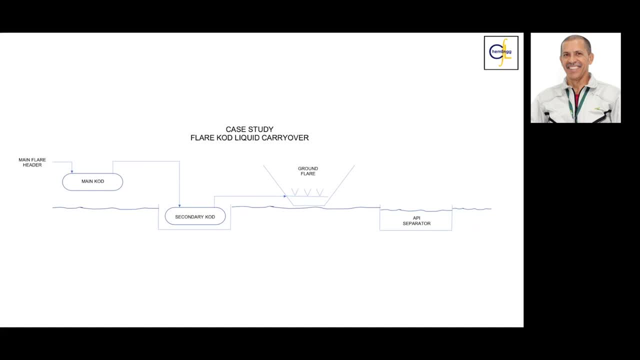 knockout drone is never on use. it's never on use, So we can allocate this volume temporarily in that drone. What happened? They bypassed the operation of the pump and they include that volume, that extra volume of liquid, And then they went higher than the maximum liquid level. 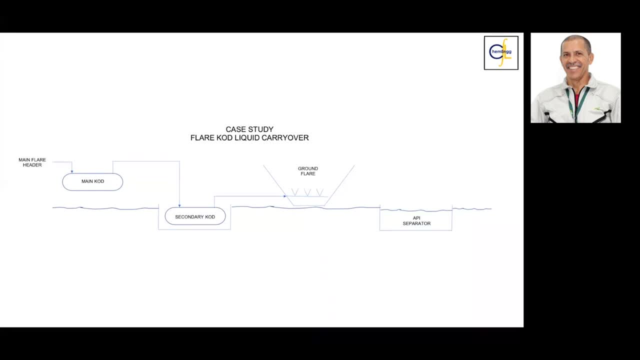 because it was a temporary solution while they solve the problem at the alkylation plant. But what happened? that there is somebody that his name is Morphy and the Morphy law So say something that expect the unexpected. So they never expected that they have an emergency there. 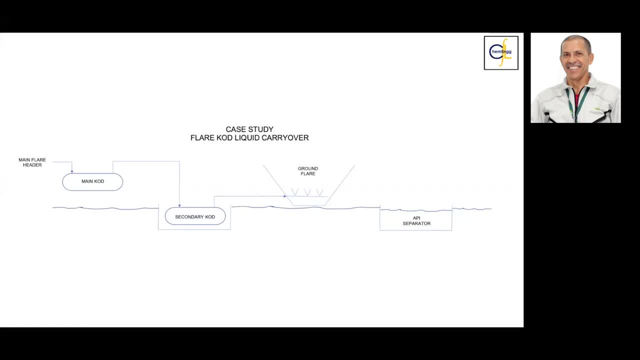 They have an emergency, a huge flow rate from here, And then this part of this excess liquid was carried over to that system And that was the real cause That generate the fire there. But of course they didn't during the contract of the study. 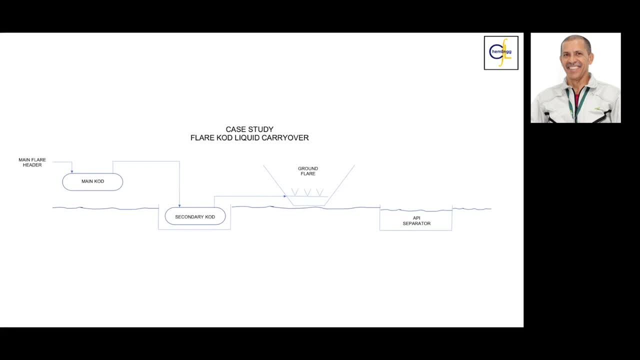 they didn't tell us that. but what the real cause? But you know sometimes, so the root cause is known When you start to run investigation so you can deal, you can find the root cause. that is one of the important issues. 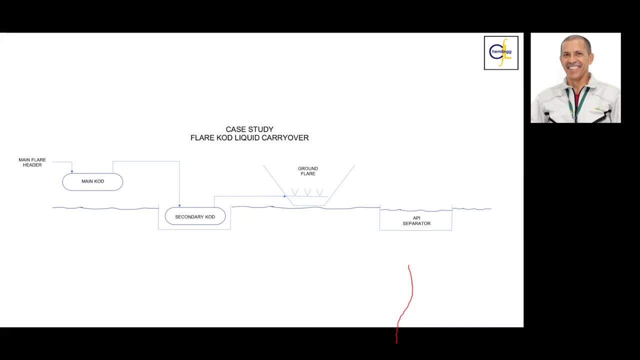 that we as a process engineer have to work as well. So not to deal with the consequence, go to the root cause, because if we solve the root cause so the consequence will disappear automatically. These things happens in any case in process plan. So when we have both of these things we can solve the problem. 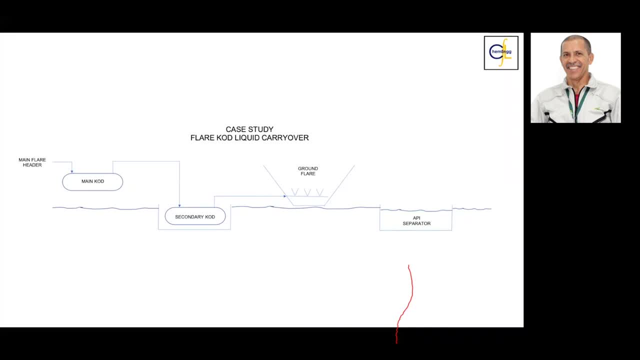 So when we have both of these things, we can solve the problem. So when we have both of these things, we can solve the problem. But we have- yesterday Mr Henry was talking about the optimization, But we have. yesterday Mr Henry was talking about the optimization- 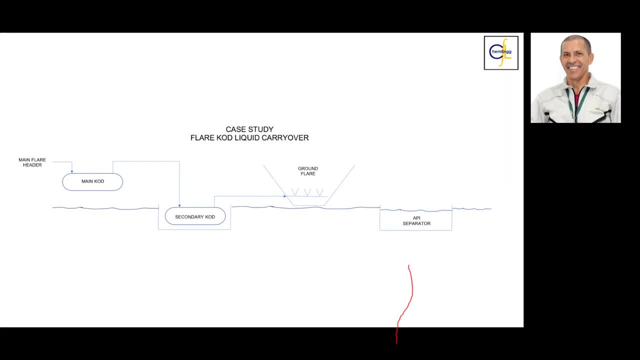 and then optimization as well. You have a root cause over there. So what do you want? Optimize a plan, but for what? What is the purpose, What is the reason? So you need to go for the root cause to get the consequence. 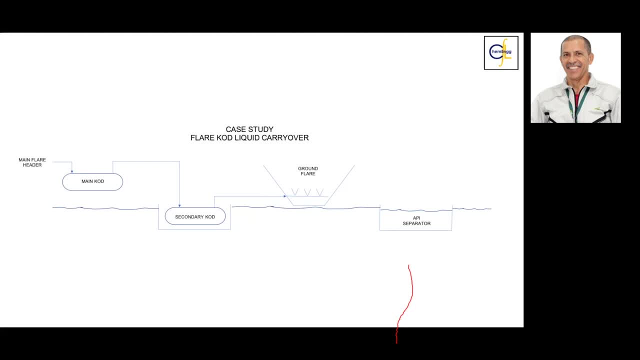 In this case, was like this: And in these cases that the- mostly the owner of the plant- is tackling the consequence. But okay, what was causing that consequence? Because when we run the analysis for all the system, we say okay, so we don't expect it to carry over. 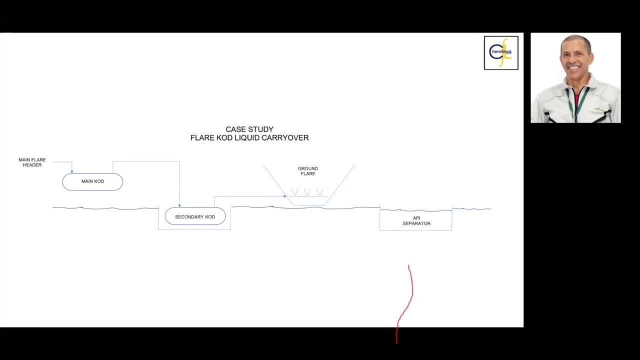 according to the capacities we are managing and the size of each drum. So there will not be liquid carry over. However, when you do this, it will not be liquid carry over. However, when you do this, it will not be liquid carry over. 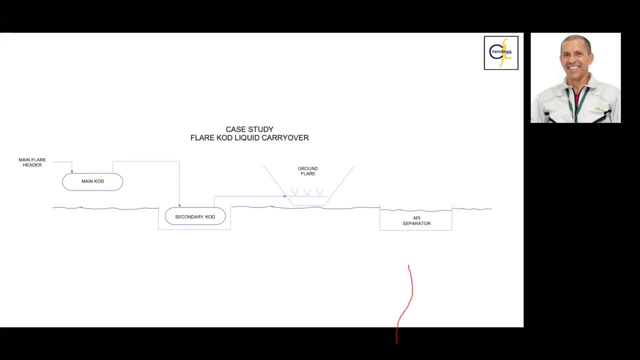 When they do crazy things, so you will get crazy consequence. Okay, and then- don't forget Mr Murphy, say something that is very clear and very real. Okay, if anything can go wrong, it will. is what he said. And then what we have to do: 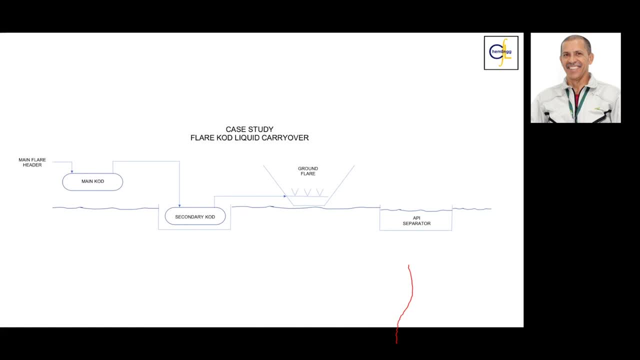 point of view, process safety management is to get rid of that principle of Murphy, is to get rid of that principle of Murphy, is to get rid of that principle of Murphy And to think with our head and think with looking for the good cause. 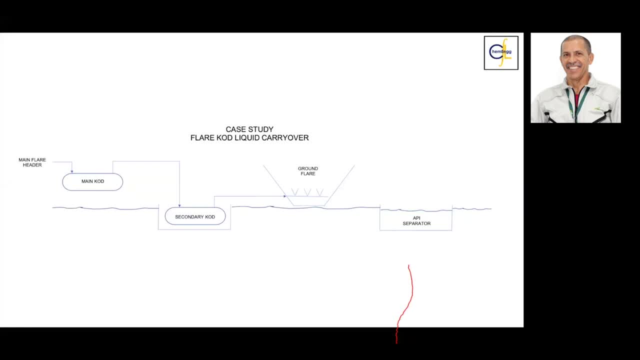 using our intellect, So using our, the principle that we learn at university. however, don't try to, don't get pushed by pressure, because anytime we are in plant operation or in business, because anytime we are in plant operation or in business, because anytime we are in plant operation or in business, 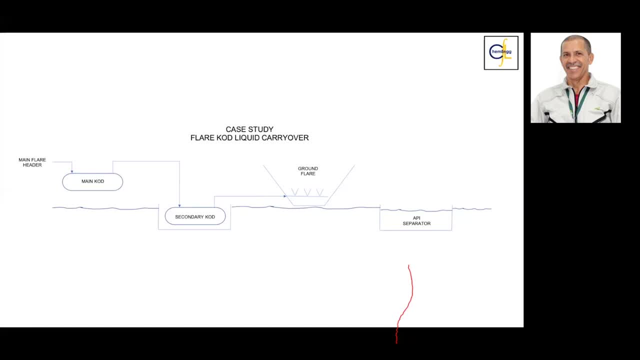 in project development development. we have a lot of pressure because everybody wants everything to be solved in less time and with low cost, And then, when you do that, the quality of the project will go down and the safety of the plant will be in game. 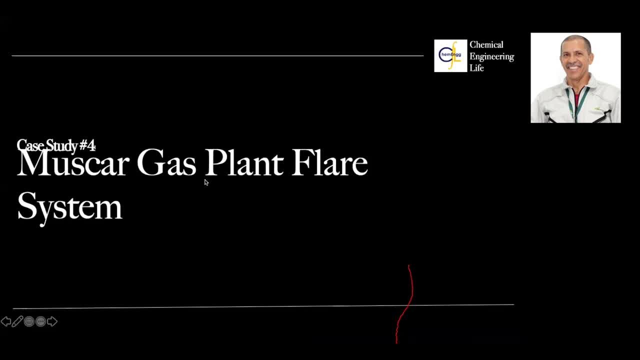 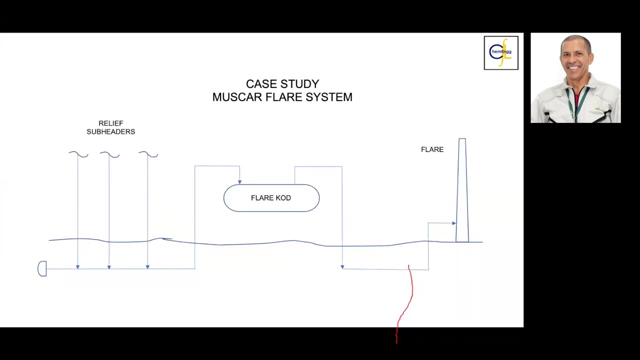 Okay, So let's go to the another, please. In this case as well, we will call for the wrong study, a safety study for the Muscar gas plant. the first system. Go on, please. And then well, I will not explain too much. 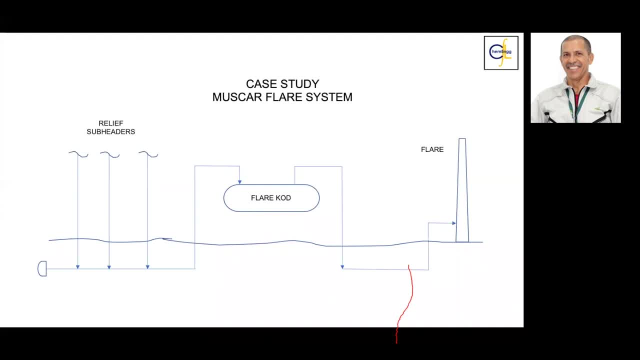 what they do in that plant or whatever. It's very important to know. So this Muscar Muscar is a very old gas plant in Venezuela And they don't process natural gas. they say They use treat the natural gas. 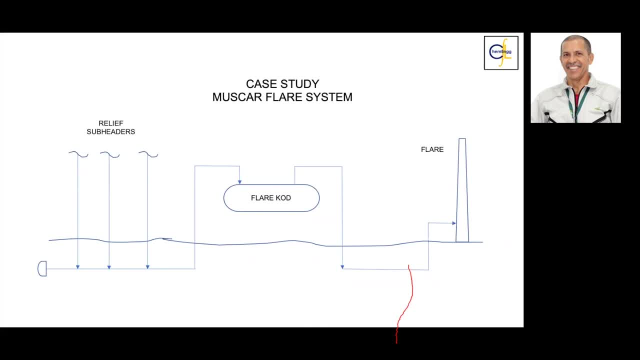 So they dehydrate the gas, they sweat the gas, they control the dew point of this natural gas. So they dehydrate the gas, they sweat the gas, they control the dew point of this natural gas, That is the natural gas for transportage. 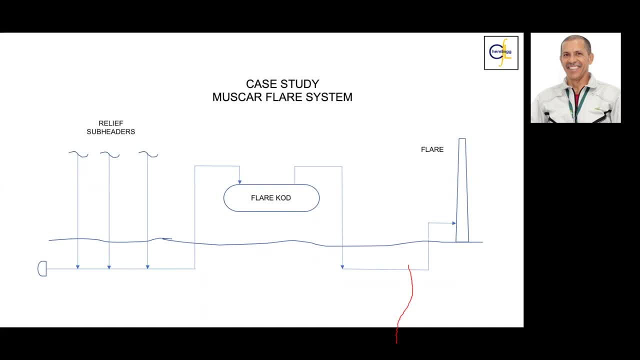 Bella, Basically is what they do in. that's the plant and already they have a re compression section to re inject, because I'm very high pressure to produce crude oil. Okay, Let's see what they do. And in fact, a long time ago, maybe in the year 4050, this is true. the gas processing was not interesting because the interest was to produce crude oil, But crude oil was the source of energy And in countries as my country, Venezuela, that we are oil producers. 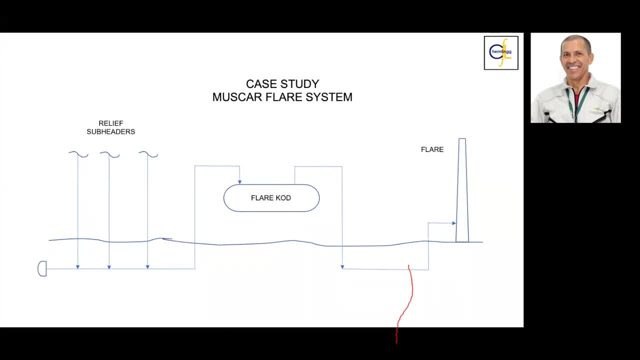 So the investment was to export crude oil to get money, And then the gas was not of interest. Now the gas became interesting from the years 60,, 70 and on, But before, so they don't mind the gas plant. And then thinking with that way: 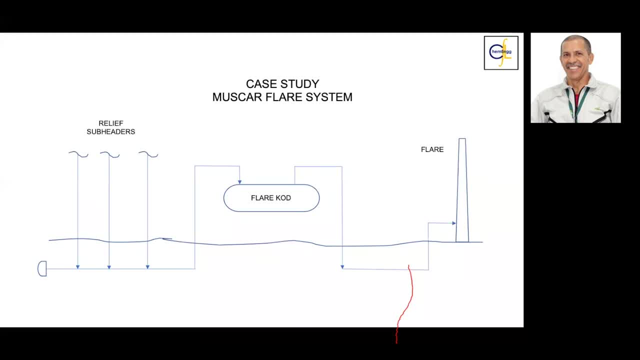 so they make as well crazy design for the gas plant. And then during that study that we run, they call us because they have the existing flare knockout drum explodes. They have an explosion of different knockout drum And they didn't know why. what was the reason? 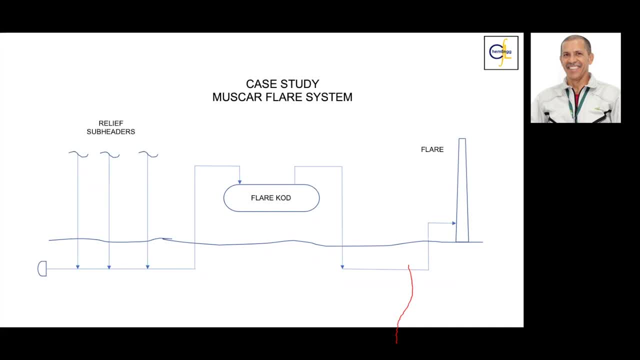 And they start to take measures. After in there they start to start to check what is the venting, the normal venting operation. So to you know, they start to look a little bit what was going on. But again they were tackling the consequence. 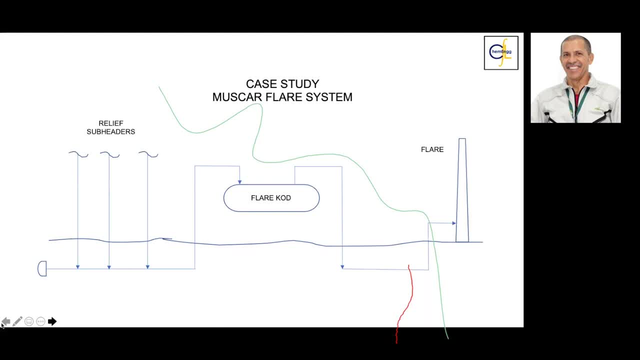 They didn't go into the root cause When we got in that plant. so we tried to understand what was going on And then this is what we found: That the main flare header was on the ground From the release of header. so the main flare header. 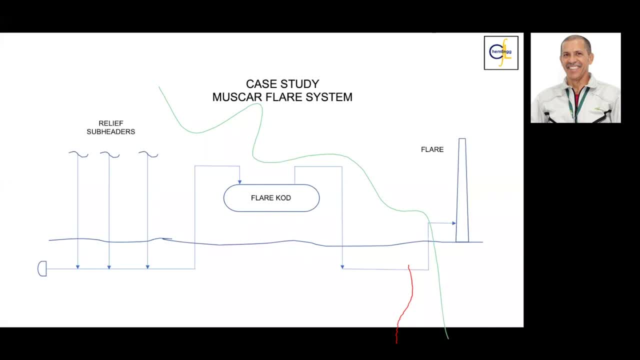 was on the ground And then go up to the flare knockout drum, And then it went on the ground again to the flare. Okay, And then what happened? when you have gas on the ground, It will condense, because normally, normally, this line: 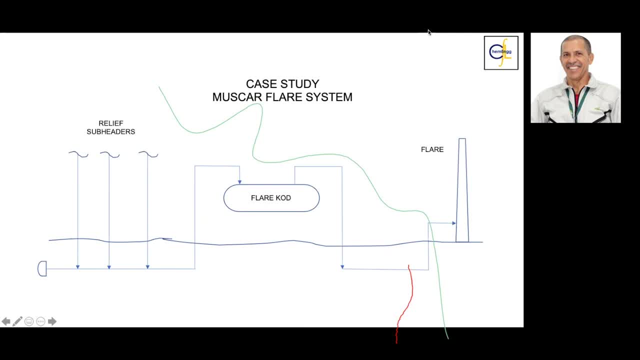 this pipeline need to free draining to the flare knockout drum, just to avoid accumulation of condensate. Same thing with this line there. This line need to be need to free draining to the flare knockout drum, Otherwise you have liquid accumulation in there and liquid accumulation in there. 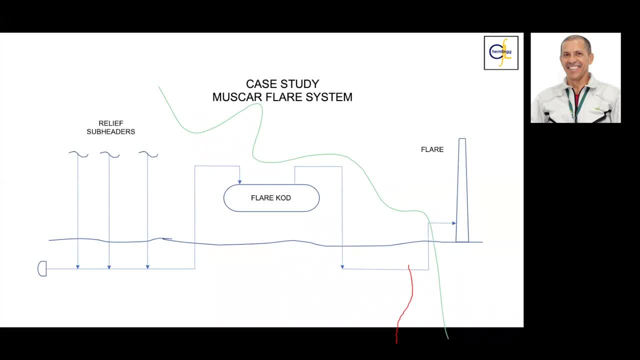 So what really happened? that there were a huge release of gases and then you have a block of liquid flowing that way that this, this knockout drum, couldn't manage the force and the impact of that block. and then the flare, And then you have another bottleneck in here. 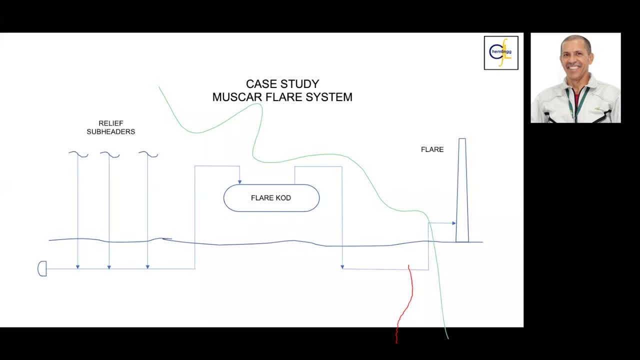 because this line as well was blocked off on liquid. And then what happened? that the flare knockout drum couldn't withstand the pressure and it explodes, Because- remember this flare knockout drum- normally the same pressure is 50 PSIG, So it's no more than that. 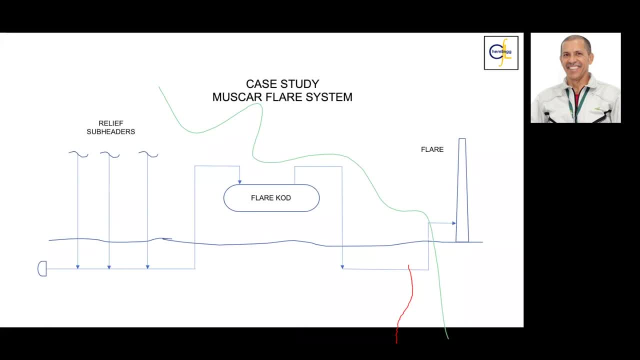 Because this is supposed to operate the pressure, But you have more pressure than the flare, And maybe we put five to 10 PSIG for this- the operation of this flare knockout drum. So the system operates at low pressure, And then. so what we found is that the most probable cause. 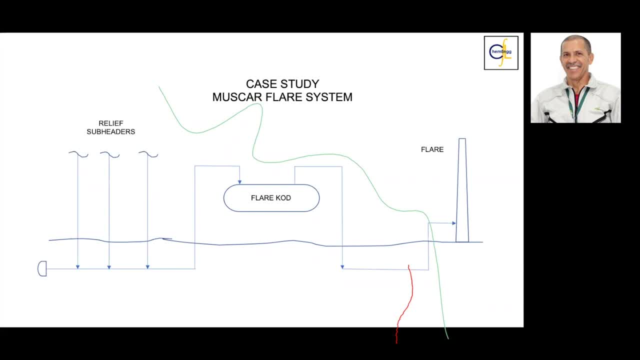 for this to explode is that you have a block of liquid in there that has been pushed for a very high flow of gas, And then the different knockout drum couldn't withstand the pressure. And then what the recommendation of this study is say: okay, so what you have to do is to re. 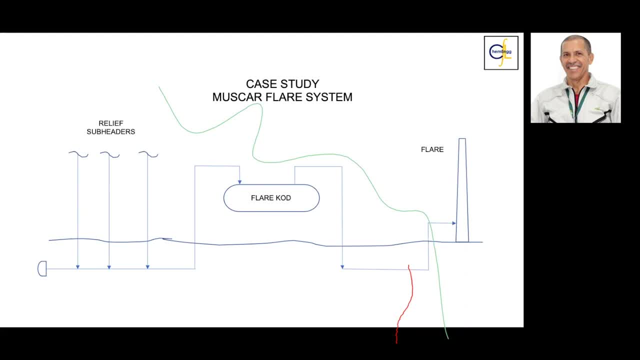 so to install a new, a new flare header, Now not on the ground but above ground, draining free to the flare knockout drum. And then we have to do something in here as well. So you have to elevate your flare, You have no choice. 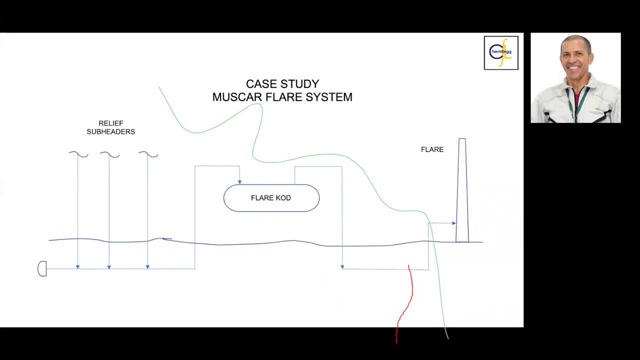 To elevate your flare to allow this line to be free draining to this, Because you don't have so, in that in this kind of system a pocket is not allowed. But, however, as I explained, so in the year this plan has been built. 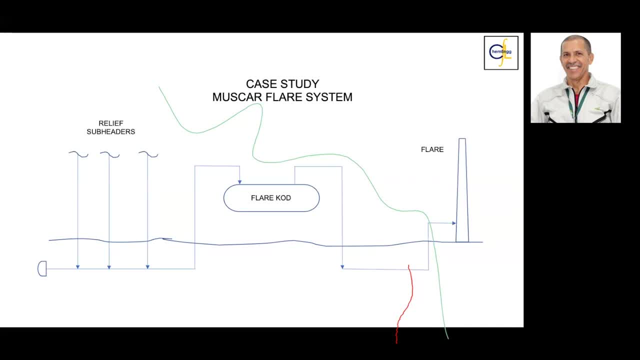 So they were not aware of the gas, So they didn't care. However, during the development on this plan, now the gas become interesting, So they introduced the hydration, They introduced gas. They wanted to introduce here NGL recovery. They want to introduce more things, but they didn't. 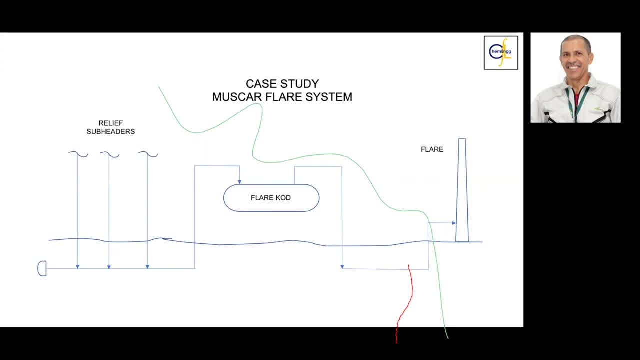 But they didn't, But they didn't. So the problem at that time and this is the consequence they have. Okay, So here in this case study that I presented- so it's most cases- for us to use what the process engineer. 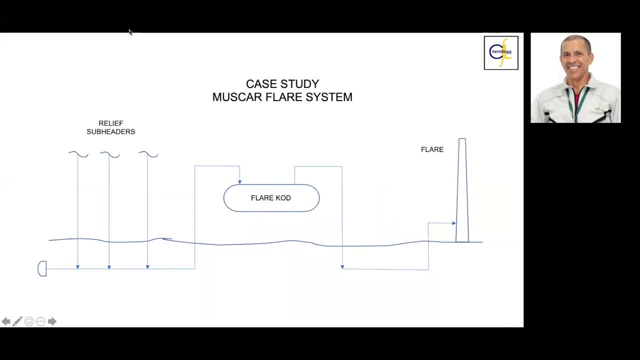 what is our role? So to design safe and operable plans and to sorry is the plan is operation and this one at the case of the validity, So we have to solve. So to go into the root code and solve the problem with the root code. 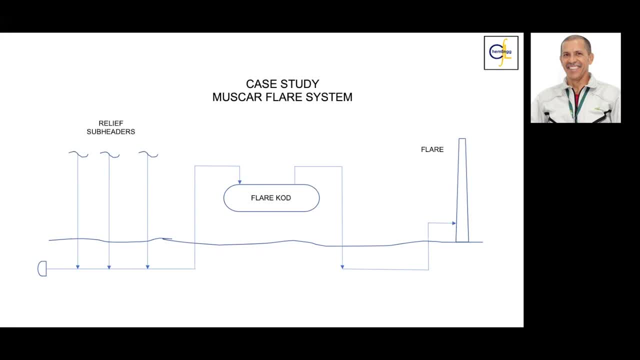 Using our common sense, using our intellect and using our role at Process Engineering, But don't think it is too easy. Okay, Because we have a lot of- I don't call- constraints. I will have lot of resistance, because most of the resistance are the operators- the operators, so they don't 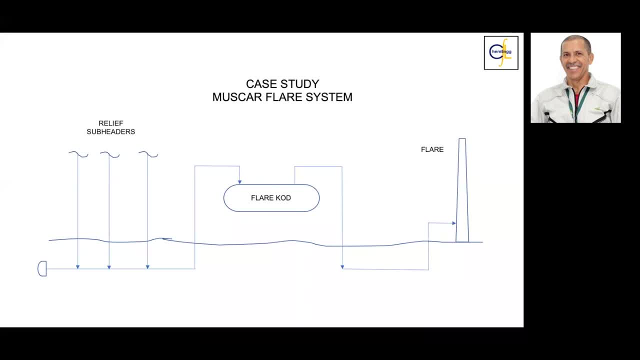 want to change anything in the planet. they want you to produce, produce, produce, produce, and they don't think most of the time, they don't think about change. okay, this is the kind of people. we need to be firm, we need to be very hard, we need to be real, we need 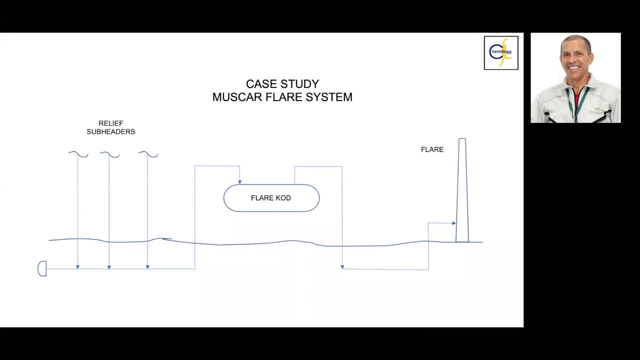 to let these people- operators and project managers, most of the time the client or the process plan owner- to let them know that process safety management is very interesting for the plant operation. okay, for the moment, this is all i have to say. i don't know if i got on time or not. 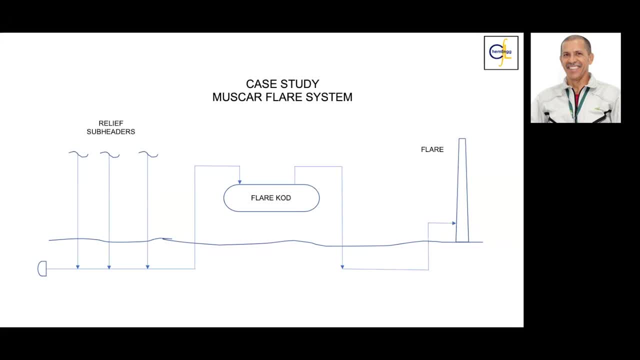 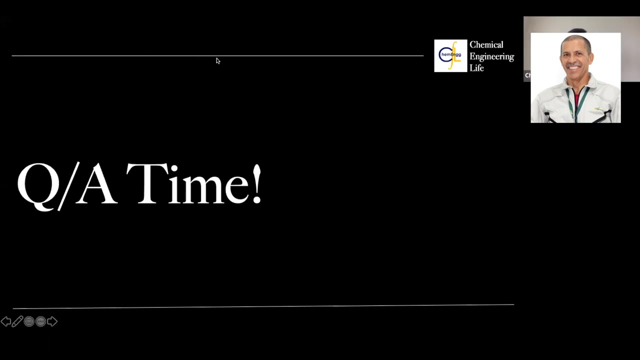 because, as i told my, my mentees, so i i speak too much because i have a lot of things that has happened during my year of experience. oh, you made it just in time. that was completely perfect. thank you, mr fredo, then. so now is the question and answer time, and the feel free to write. 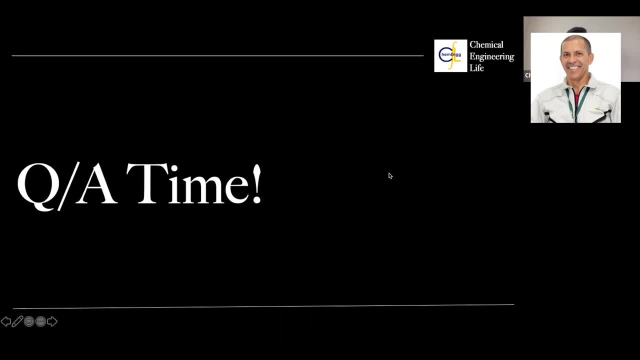 the course your question in your chat if you want, or you can also unmute yourself if you would like to ask questions. hi, sir, hello, yes, hello, uh, yes, yeah. so i have one question regarding this. uh, muscar, a gas plant player. so, uh, as we saw, the player header was going from underground. 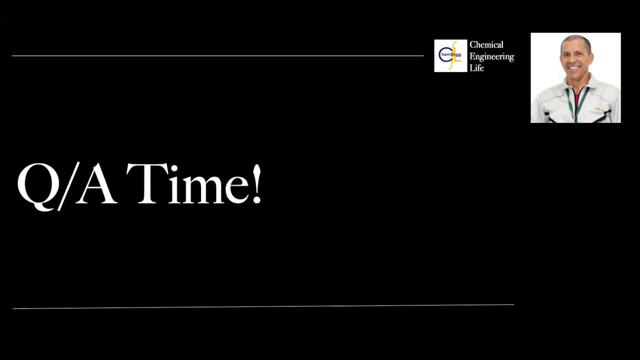 originally. uh, why was it so? so why they made it go through underground, like usually we don't see that right in which. in which system? the muscar, muscar gas plant flame? uh, you mean the the one of muscar plant? yeah, right, right, right, yes, stereo. so why was that flare header was, uh, designed to go from the underground and not 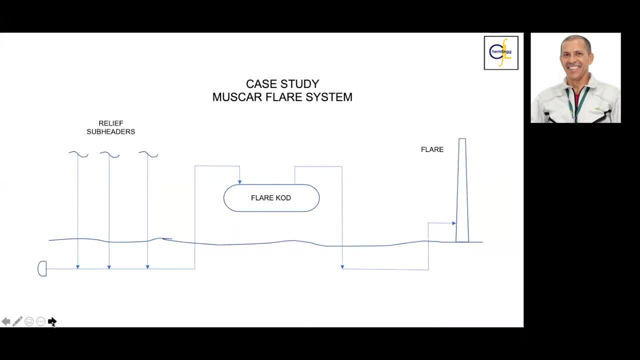 from the overhead above the ground. no, because, as i told you, so it's a, it's an uh old plan. uh, they didn't, they didn't uh care about that. and then they built the plan like this most, most. if you go to feel for the old fields, let's say, you will find a lot of underground. 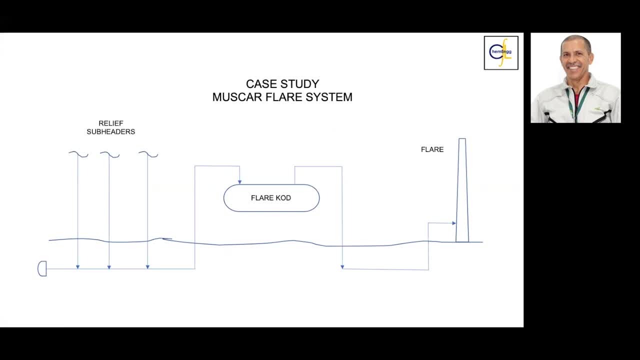 pipelines, because this is the way, the easy way, they found uh to build process plants. however, this is the thing that we found, and then the recommendation was to uh to get rid of this on the ground plan and to install a new, a um, flat header, a above ground with uh, a free draining to the pleno caudron, as it should be. 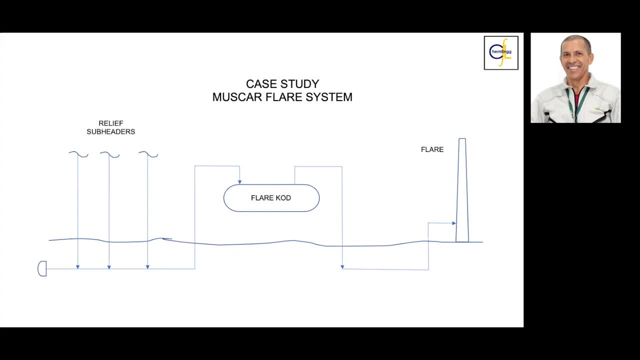 okay, thank you, sir, thank you, thank you, okay, thank you. so so my next question, so my next question is the one we said about flare kod liquid carrier, in which one a flare kod liquid carryover and the liquid carryover. okay, what is the question about there? uh, sir, uh, was it possible, uh to you know, install a? u piece there, uh, between main kod or? 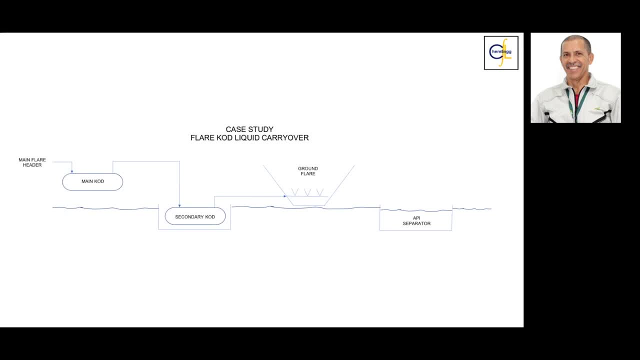 secondary kod and between secondary kod and ground ground pair so that whatever liquid was you know, carryover was happening there. that can get uh settled down, yes, but uh as, uh, as this system has been sized. okay, it has been designed so the the um, this main knockout drum is. 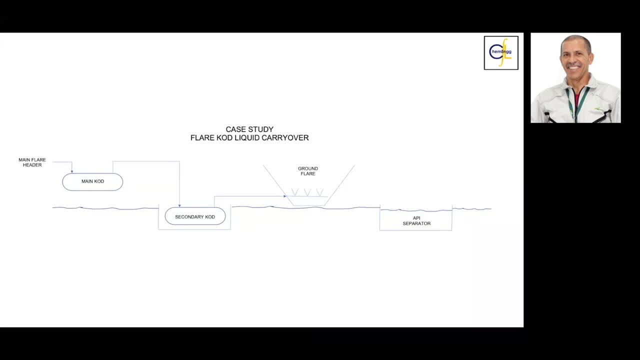 the one that will receive all the liquid. this secondary kod is to, let's say, to receive the potential condensing a hydrocarbon from this line there and from this line there. that's the reason why this secondary knockout drone is in a peak- okay, as you see there. so this, this represents a. 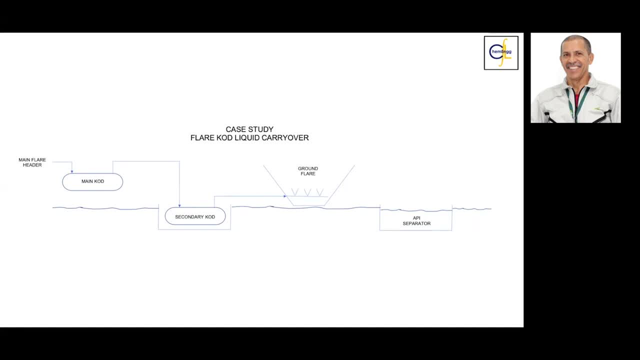 peak it is below, is below ground and this uh byline in here is uh free draining back there. okay, to avoid, precisely to avoid, liquid in in this, um, in the ground flare. however, uh, the liquid carryover was for an another reason, because when we run the evaluation of the friend of cow drum for this one, on any of these, of the friend of cow, 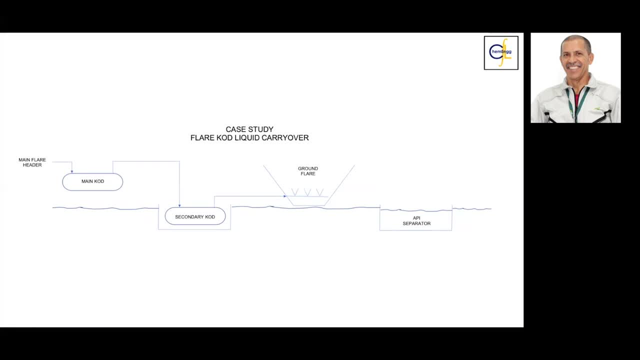 drum in the plant. so we haven't found any anything in any problem with the liquid carryover because the, the, uh, the drums were or was or are- because they are already installed and in operation- big enough to manage any condensation liquid. and then the pump system. pumping system: there was big enough. 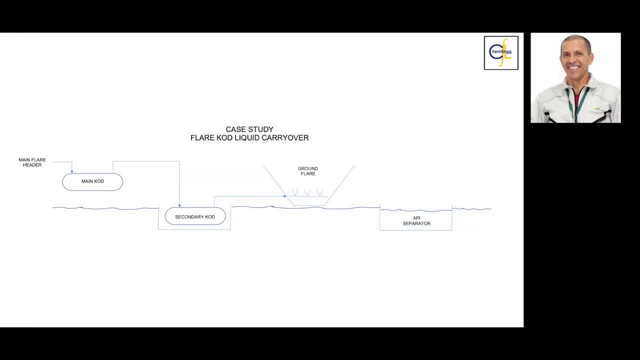 as well to take that uh to control that quantity of liquid in the. uh, those knockout drop okay, okay. okay, got it. thank you, sir. however, the your question is very interesting. this is another case study i have got in another plant during design because you can design in that project they- it was a. 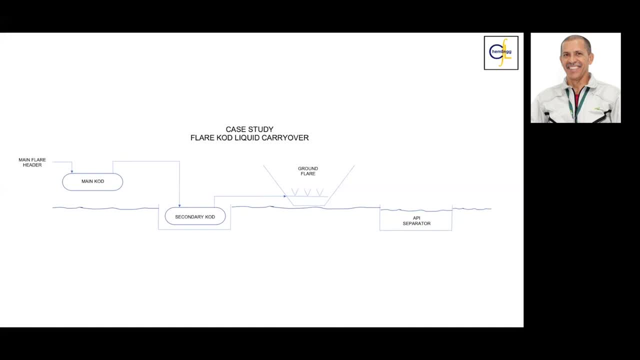 ground flare as well. however, this secondary knockout was not there, okay, and then they have the main account that was elevated and this line go like this: to the ground flare and i say, perfect. so i like that, i like this system. tell me how we get free of condensation in that pipeline to where we will send it. so who will collect any condensation? 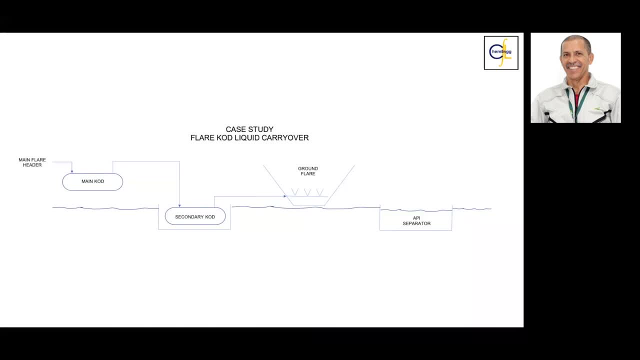 in this pipeline is this knockout drum is at a higher elevation than your ground plan. and then i let just that question to the, to the management, to the project management. so let me know how, what we will do with this, because this is a big problem. unfortunately i have to. i left that project before the end. 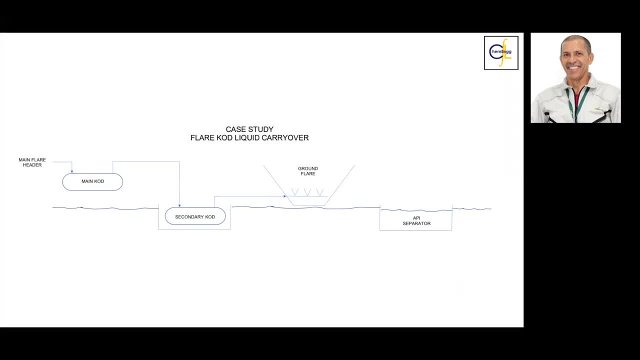 because i don't know what was the solution. define a solution for that. because they didn't want, uh, any pit in that project. say, okay, they didn't want elevated flare, they didn't want a uh, a uh to build pits for another drum. i said, okay, but now we have a problem. 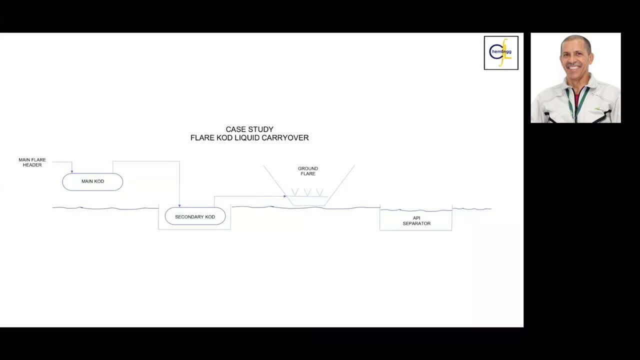 how we sort out the problem. but i never got the answer because i left the project. all right, thank you very much. okay, thank you, and we have another question um that: why do we put flare system instead of refrigeration cycle to condense all the vapors that are coming from the source, instead of wasting them in the 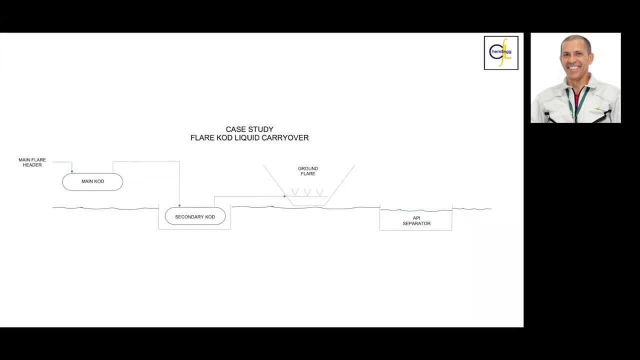 flare system. well, the recovery system has been introduced in the latest 90s, so it didn't exist before. yeah, i have a question. so uh, now, nowadays, so, uh, most of the owners of plants are thinking to recover, uh, the most of the liquids for the flare gas, because we know that the flare gas is a rich 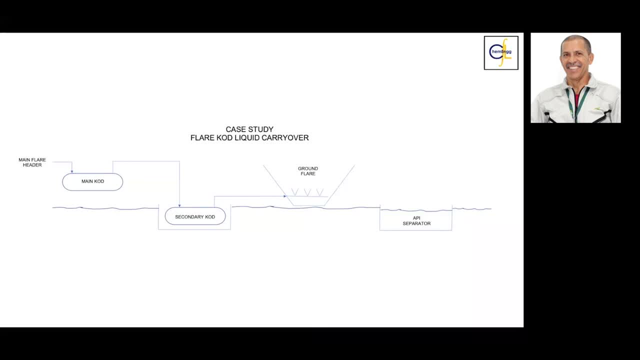 plane, so you can. you can get a benefit for that forecast, but remember that we as well, so we have to to invest in that, this recovery plant that most of the owners don't want it, so the best idea is the If you are dealing with a new plan. 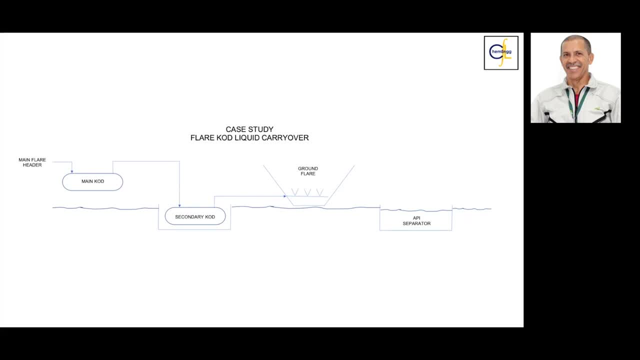 or you are dealing with an old plan but you are working on revamped plans, so try to introduce that idea during the evaluation of the cost of the project. Don't do it after, so do it before When we are discussing the scope of the project. 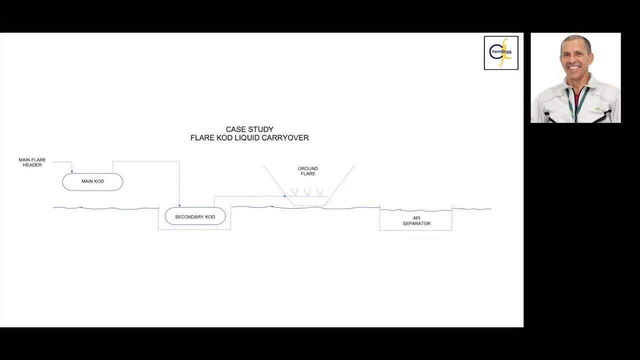 so to introduce that idea, to be so to try to get one approval from the owner of the plan, because at the end of the day, it's more, because it's the cost. I have seen this system as a recovery, but not in FLAIR system yet. 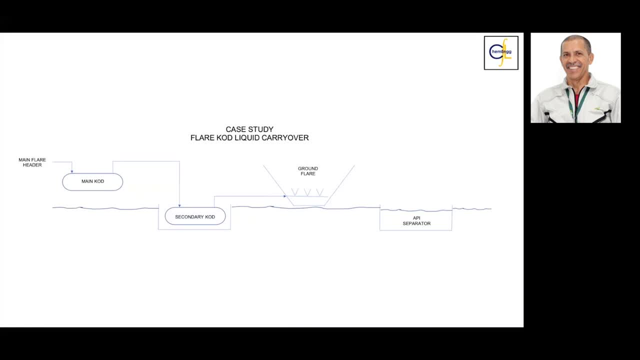 I have seen it in papers, in magazines, but myself I have not seen it in a plan in operation. I have seen this recovery gases in another plan, for example, when the loading or uploading chips with light products as methane or propane. 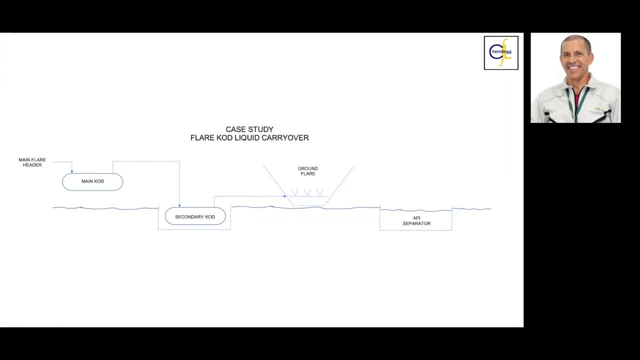 So you have the gas recovery system over there with the refrigeration, But I have not seen one system you know, but I have not seen one system you know, but I have not seen one system you know in operation for FLAIR. 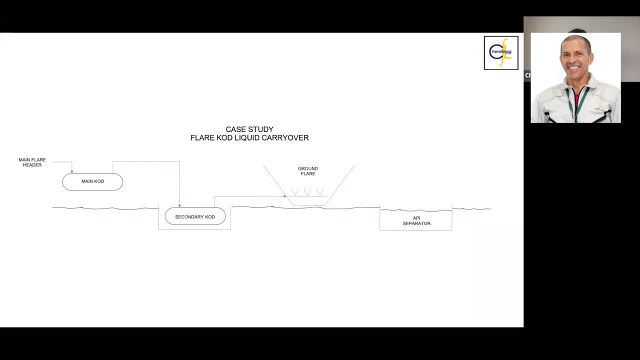 Perfect. Thank you, Mr Vilfredo. Are there any other questions? Please feel free to unmute yourself or write them in the chat. Hi, one more question. So what was the criteria for bifurcating in the first case study? 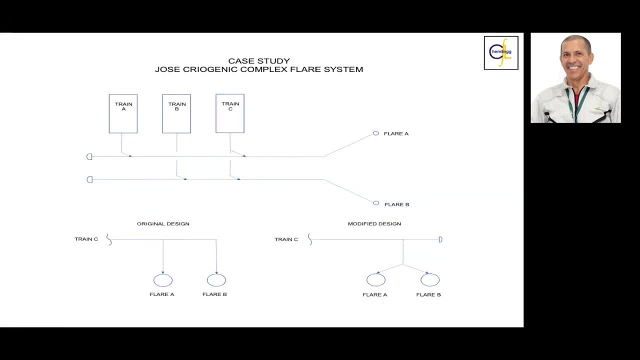 sorry, what? how did i get a phone? by forgetting that fluid for drain c? so you mean you mean this: yeah, right, right, flare c. no, it's, it's. it's not forgetting that. i think that it's more a lack of experience. okay, dealing with this. okay, it's not, it's not forgetting it's. 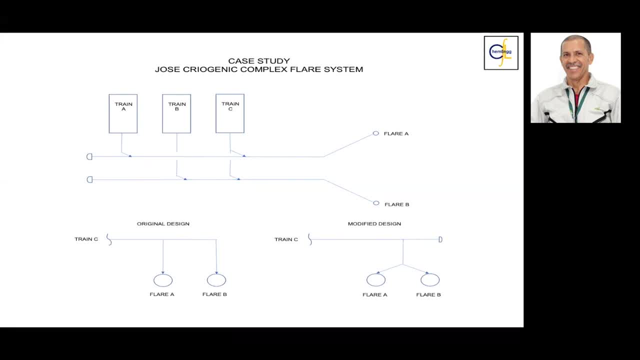 from my point of view, now that i am seeing this in cold, in a cold site, it's lack of experience, so at that at that time, so we didn't figure out that. however, a um, i have seen another systems, a cooling water systems. it was a cooling water system that it has. they have the same, a similar. 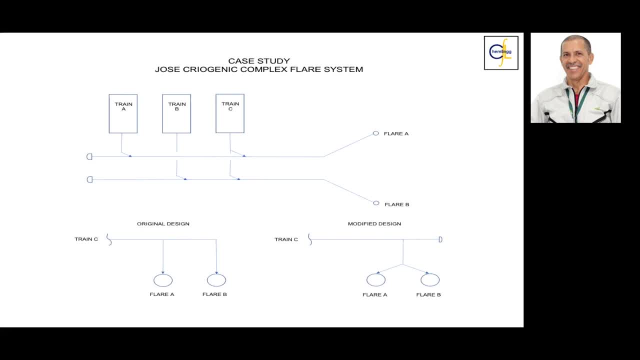 problem. they have a couple of condensers, okay, a couple of condensers, very, quite big condensers, and they have a bad distribution of water in this condenser because the arrangement was like this. okay, and then what they did to try to control the system? is they closing the valve? 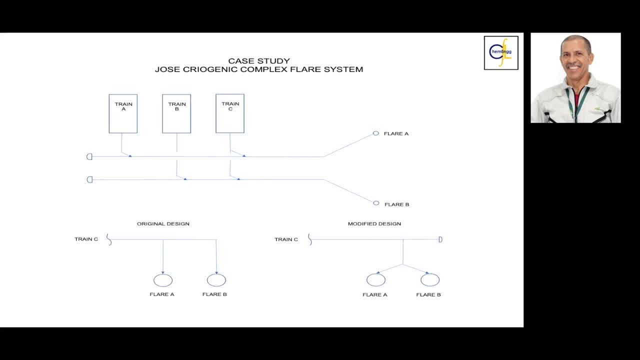 manually of one of the system to get more water into the other condenser. okay, and i say okay. so this is, this is, and this is what i realized. so this is a bad design. if you are looking for for a very good distribution, we have to do something. and then we face that. 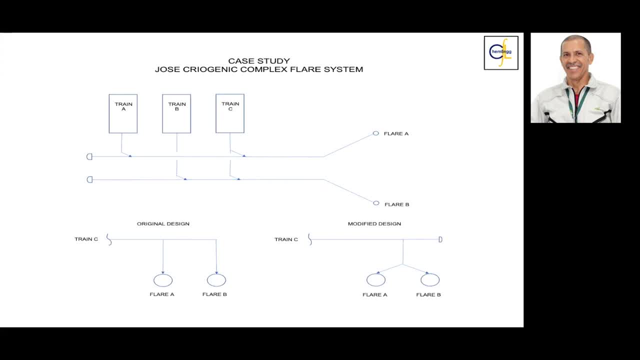 in the tracy. i say we have the similar situation for different systems, and then this is the reason i i am talking about fluid, so not talking about gas or liquid. so what we need to do is to create a water concluded system in order to guarantee it is a good distribution of the system. 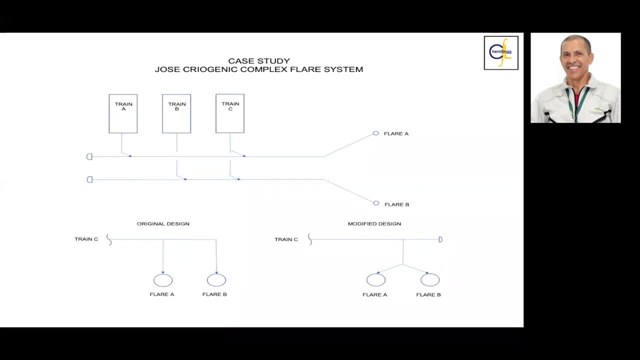 because when we run uh simulation, the simulation will tell us according how. how do you have the return in the case of cooling water? how is the arrestment of the return? it will tell you what is the distribution. it is fine point of the simulation, but when you go to the reality, distribution is only that. 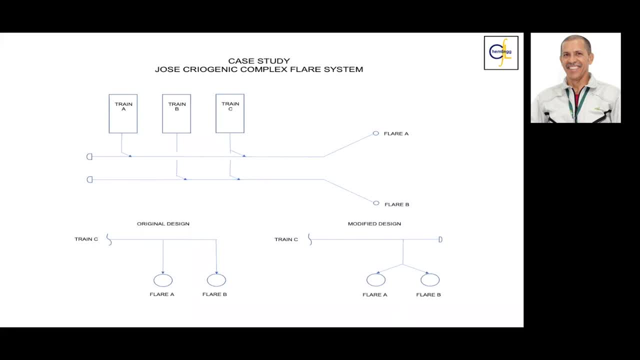 to improve the flow distribution of this kind of system, Not only in that case but in other cases as well. So you go to old plant or old refinery that still deal with a cooling water system for the condenser and cooler. So you will see lot of arrangement like that. 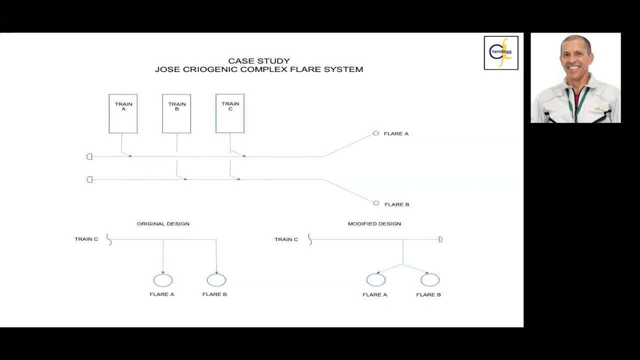 And then when you start to talk to the operators, they will start to tell you what the problem, what distribution problem they have. Okay, It's a matter of design. Okay, So it's a matter of design. and then we have to improve the design. 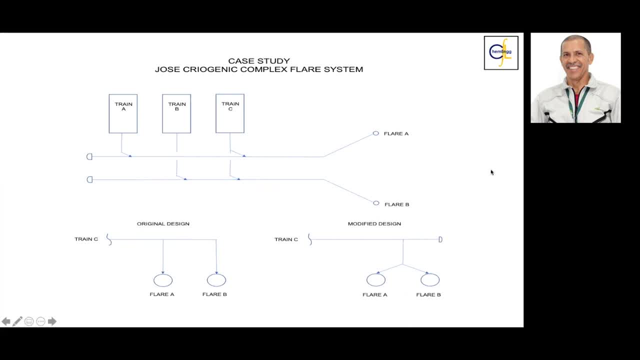 Sometimes we as a process engineers, so we need to go into the piping as well. Right, Okay, Got it. Thank you. There was a question. Can you share this PowerPoint for future reference by mail? Yes, We will share the PowerPoint. 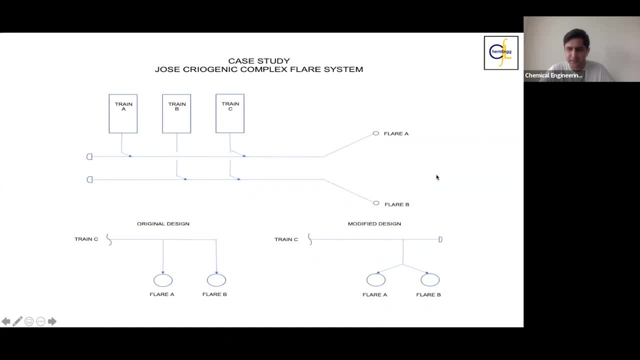 with all the attendees afterwards, So you will receive it. How many FLIR headers can be connected in a single FLIR stack? That depends on the capacity. So you have several issues in here. One is the capacity of the FLIR. The second one is the coincidence of the scenarios of these FLIRs. 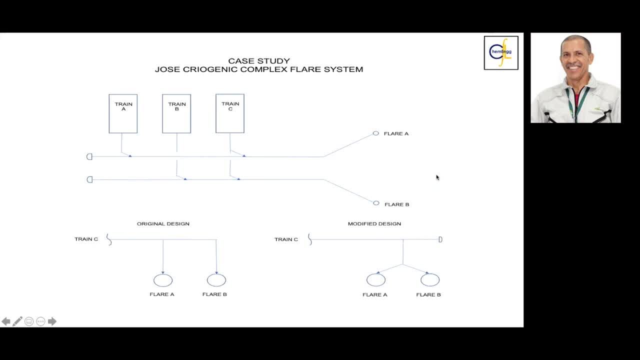 So you have to. first of all, what you have to do is to analyze and to evaluate the scenario that you have for any, in this case, for any train, for any piece of equipment. What scenario is the one that is giving you the most? 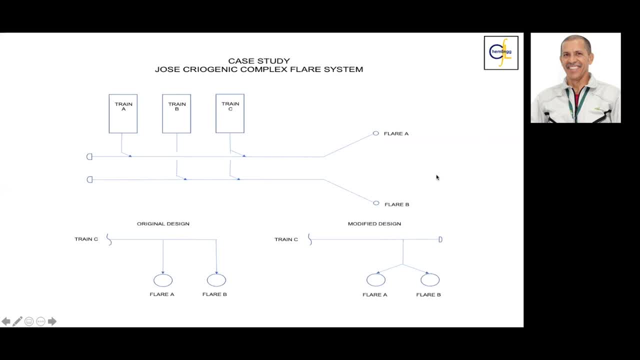 or the higher flow rate. According to this, higher flow rate is for the new size, the FLIR header and the FLIR itself And then the FLIR. you don't, you don't normally, normally you don't, you don't set the FLIR. 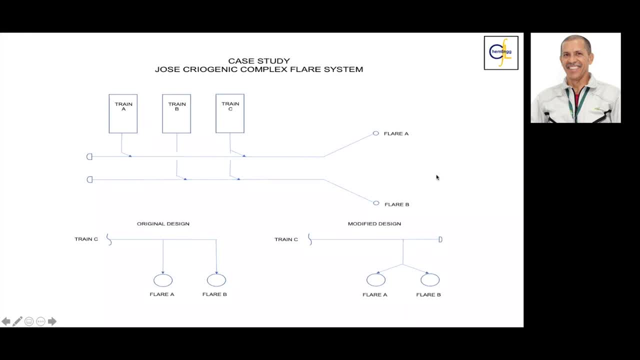 for the maximum capacity of this You will mostly so. you talk to the FLIR manufacturer and the FLIR manufacturer most of the time they have FLIR for, let's say, for capacity, they don't tailor made a FLIR for you, for your plant. 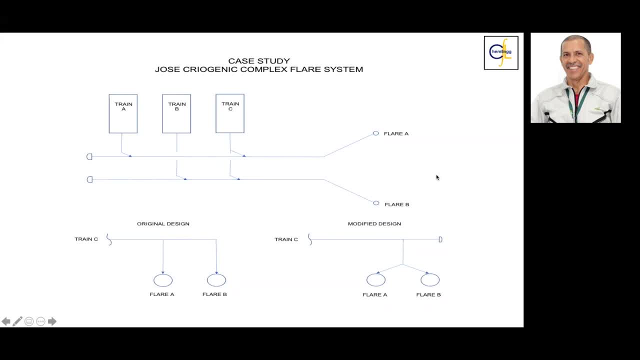 So they say, okay, you want. what is the capacity of your plant, of your plant? 30,000 barrels per day. okay, for 30,000 barrels per day. so the FLIR, is this what you need? 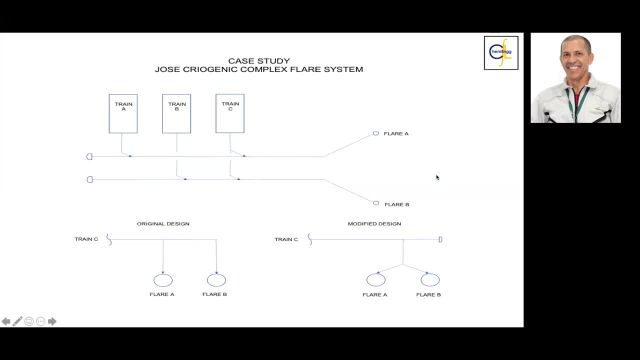 according to the capacity of your plant, Okay, and then, most of the time so you go for a FLIR with a higher capacity than the flow rate you, let's say it is required to be relieved from your safety valves and the antidepressant system. 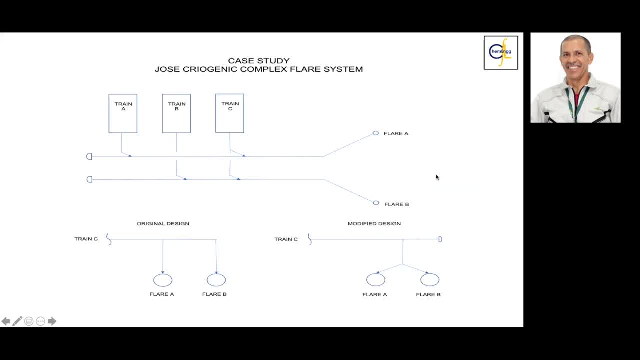 Okay, and then this is the, let's say, the gap that you have to play with the FLIR capacity, and then you can see how many FLIR can be installed in that case. In the case of ground, FLIR is a little bit more easy. 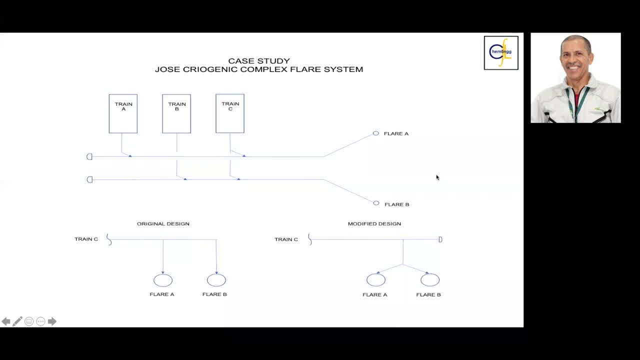 because the ground FLIR is divided into sub-burners. let's say You have a main header that is in there, but you have several, several burners, And then you can, when you have purchased the ground FLIR. 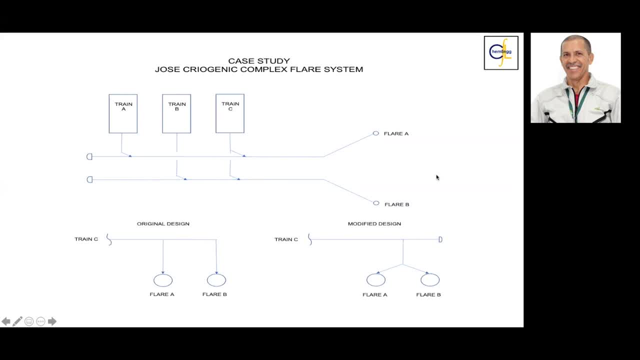 so you purchase it with spares or with, not with spares, with places to allocate for another sub-header for burners. Okay, And then when you see you may have, maybe for the capacity you need four sub-header for burner. 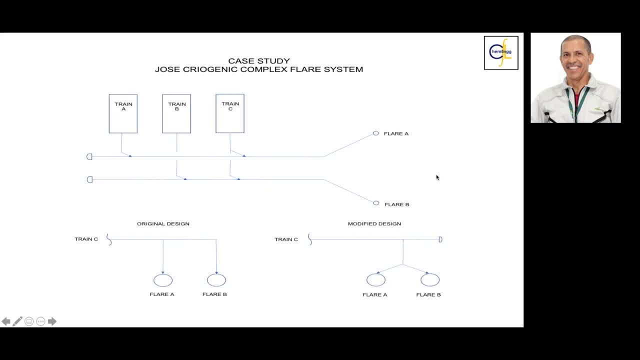 or you do talk to your FLIR manufacturer and you say, okay, I would like to. I am thinking in an expansion, I will need more capacity And then he can leave three or four more spaces to allocate for another burners. So for ground FLIR it's more easy. 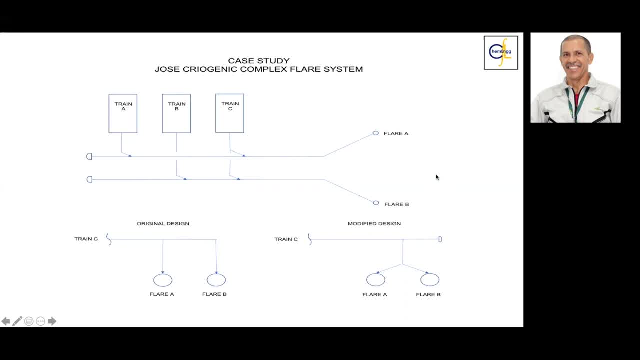 For elevated FLIR. so it's not that easy, Thank you. So then there is one more question from option. If I understand well, for emergency cases it is better to release the pressure of DC3 to a separated header to prevent overload to FLIR header system. 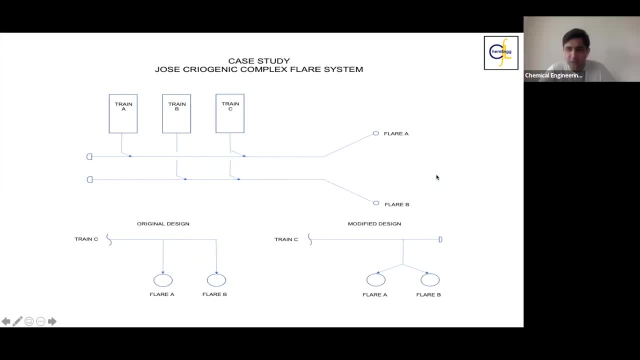 Can you say again If I understand well: for emergency cases, Can you say again If I understand well: for emergency cases, it is better to release the pressure of DC3 to a separated header to prevent overload to FLIR header system? Not necessarily. 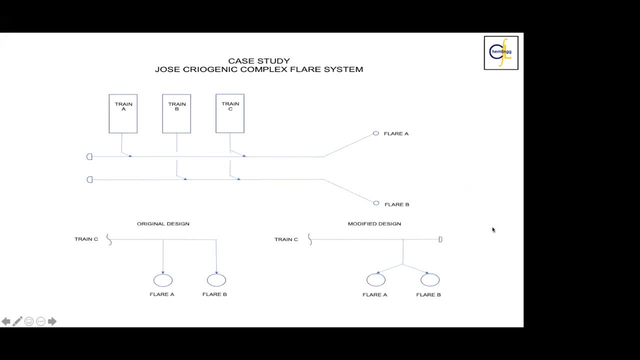 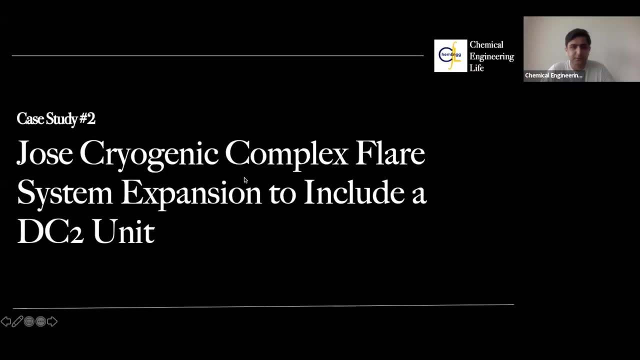 Not necessarily. I'm not sure if the question is talking about this system or the other one that includes the DC2.. I think it is this one. I think it's this one Because our proposal was this, So this unit, because 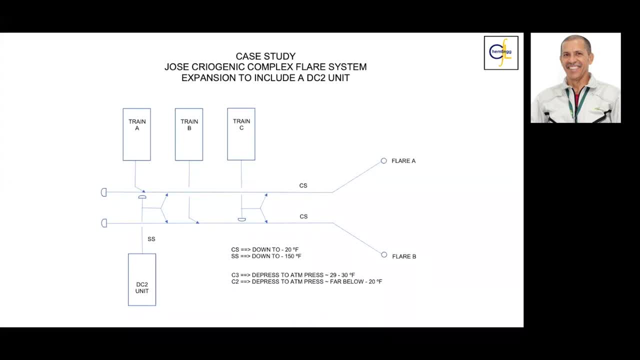 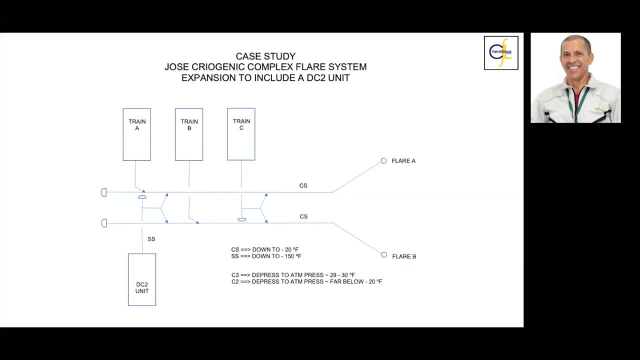 not to use the existing one. The reason was not capacity, The reason was material selection. That this system may fail when facing temperature. that this system may fail when facing temperature. that this system may fail when facing temperature far below minus 20 degrees. 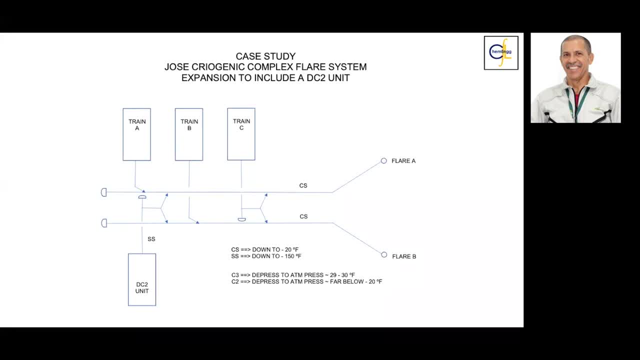 far below minus 20 degrees. I'm not sure if this is the question. I'm not sure if this is the question. I'm not sure if this is the question. Mm-hmm, Mmm-hmm. Oh, I think it was. 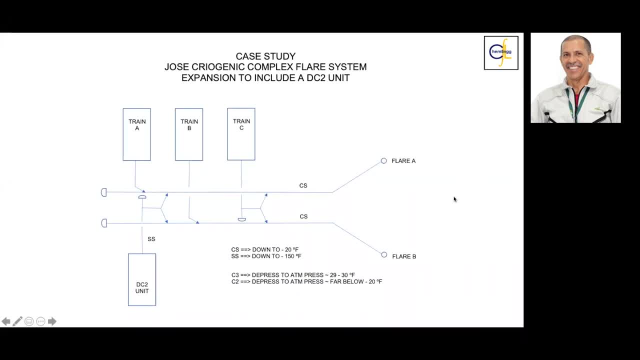 Yep, If you- Oh, I think it was yep, Thank you, But, however, however, be aware of this because I have another cases. Another case, So be aware when you run simulations of this kind of system, Because I have been auditing one technical audit. 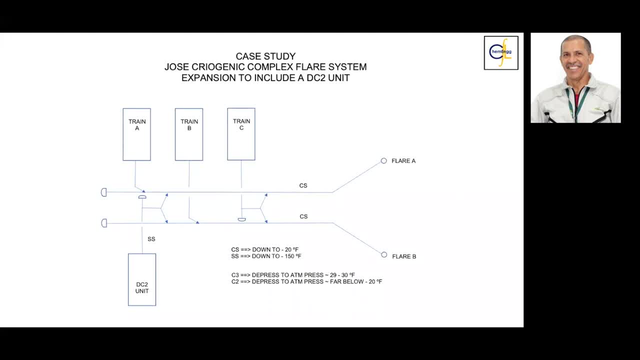 Because I have been auditing one technical audit for one DC2 unit. And then in the FLIR system they say that somewhere in here, let's say, they change from stainless steel to carbon steel impact test And then the knockout drum that was somewhere there on the FLIR was selected from that material. 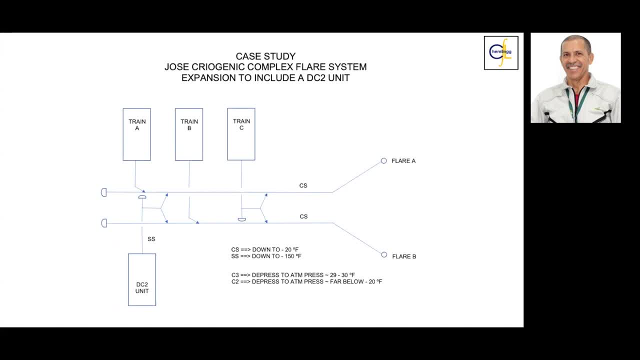 And then they say, well, from 200 meters from here to there, you change the material. Why do you do that? No, because we don't have simulation. and simulation say that the temperature in here, well, according to the atmospheric temperature, et cetera, et cetera, et cetera. 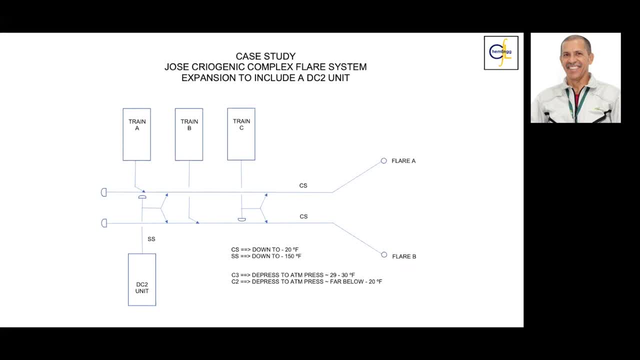 I say okay, but are you sure that at 200 meters you will have this temperature change? Because it's a result from a simulator And the simulator is giving you, let's say, some idea of what is going on, But the reality is saying anything different. 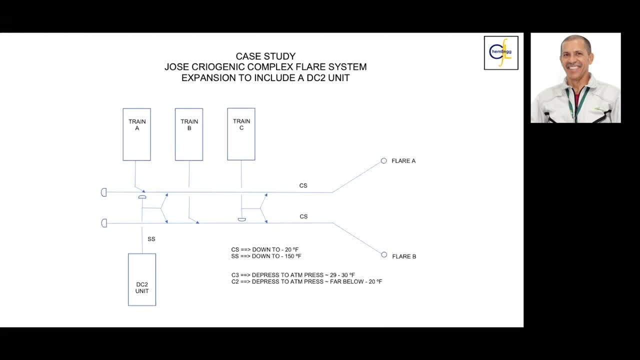 And then the recommendation in that system is: no, no, no, forget about the carbon steel impact test. Design everything for stainless steel. And then they say, well, but it costs more money. blah, blah, blah. Okay, but we're talking here about anything else. 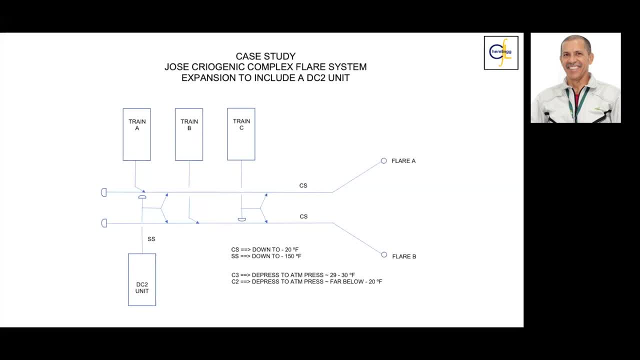 If you want to do the things well, do it well up to the end, Because simulation. But the reality is that the environmental temperature is very. for example, in countries that you live in, in Denmark, it's very cold in winter and very hot in summer. 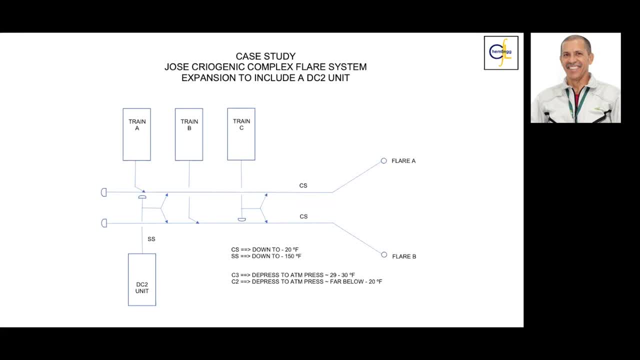 For the countries, that's our in Venezuela, we don't have this temperature change. So then you have to. you have to size everything for a very hot temperature And I think that in places like India and like Pakistan, that is very hot. 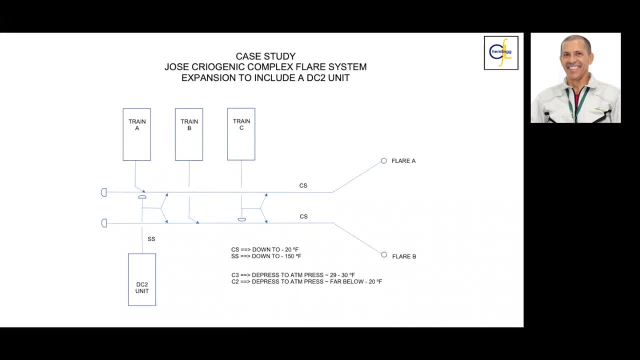 But in places like Brazil, places are well, they do the same thing. You don't think about lower temperature, You think about higher temperature. Higher temperature is another problem, But lower temperature is only seen sometimes at night. but at night it's not as, as they say, as critical as, for example, in people like in countries like Russia, in countries like Canada and things like that. 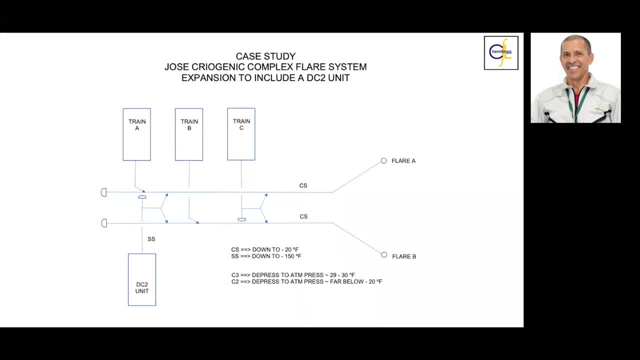 Good morning. Okay, so we need, we need to think about that and to use our common sense And then to don't get so difficult to simulate that I think you know as one one to say one idea, what is going on? 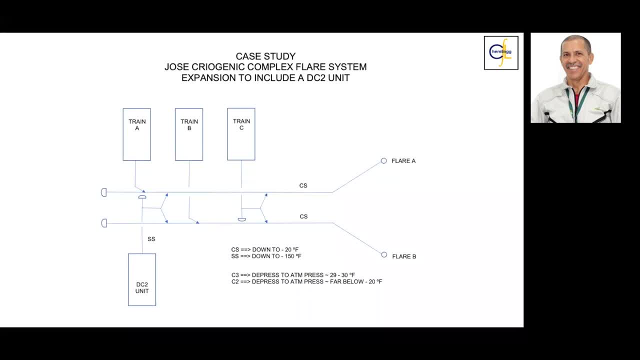 One trend, one tendency And then. but the reality is different. Because when you try To reproduce The, the plan in operation with the operations, The operation, the plan in operation with the operations, with the simulation model you have, you will never get that because the reality is different. okay. 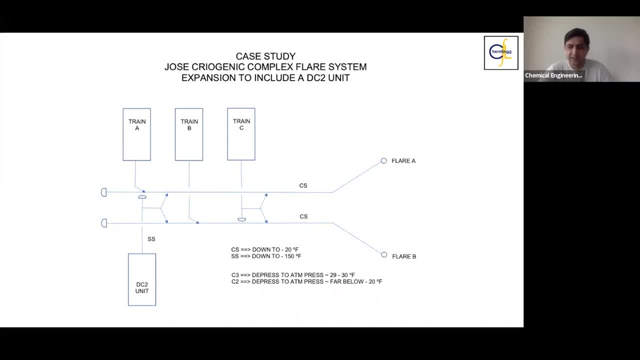 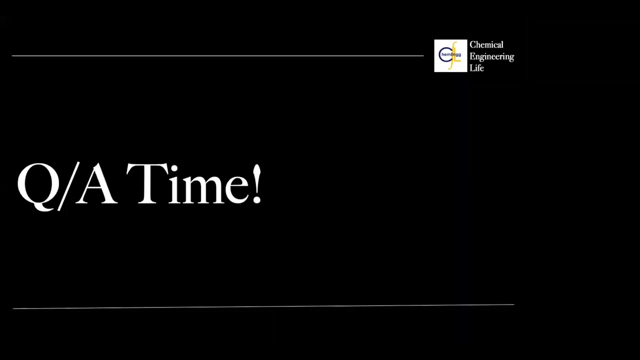 perfect, thank you, that's a very good point. thank you, so any other questions that anyone might have? if not, then we can move on to to um. i have seen that somebody else was asking for my um linkedin. oh, yes, i don't know if you can supply it. you can supply it email. i will right after the webinar. 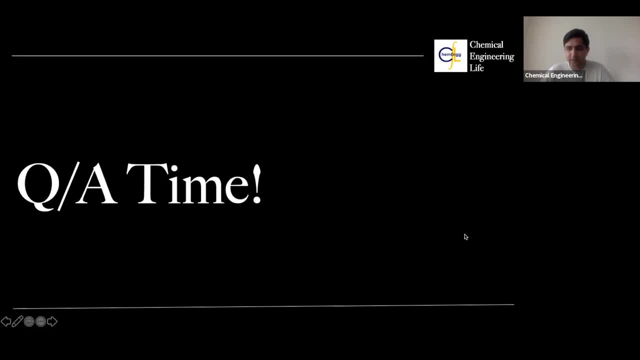 when i send out the certificate to all of you with the powerpoint, i'll also share mr bufretto's linkedin link as well, so you can click on it and connect with him there as well. so i i will do that. i'll do it right after the workshop. 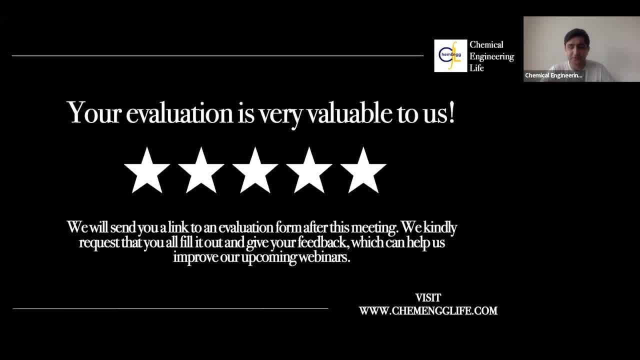 great, then, uh, about the next steps after the workshop. well, firstly, thank you to everyone that joined in today, on this sunday morning, uh, and we hope that you got something out of the webinar. now i will send out the certificates to all of the attendees with the, so you all can have a copy. 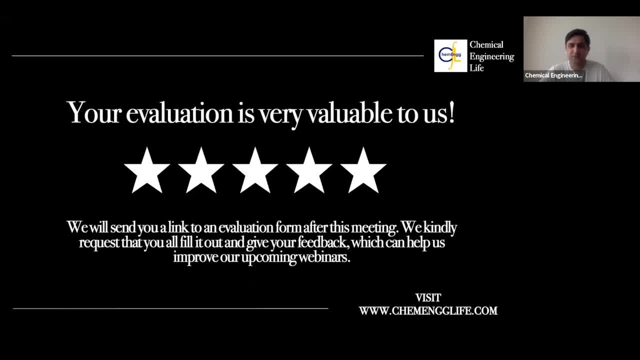 and show your attendance, if required. at the same time, i'll also send you a link for uh evaluation for the webinar and we would really appreciate it if you could go in and tell us a little bit, tell us, about how you thought the webinar was, so that we can use it to to improve. 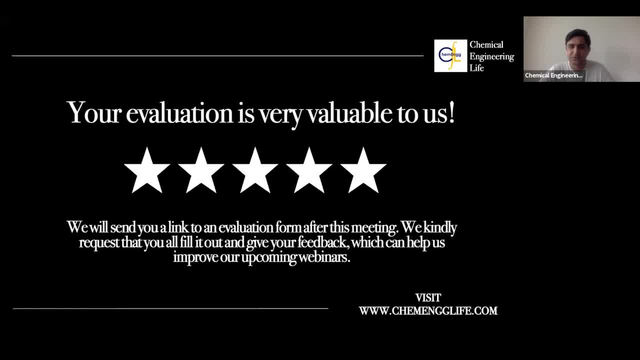 our future webinars. and lastly, i'll also share the powerpoint and also the other information and also mr lucretta's linkedin profile link in the email and also i'll also share the recording of the webinar with with all of you so you all can go in and watch it again if you wish. the the video will be out soon. 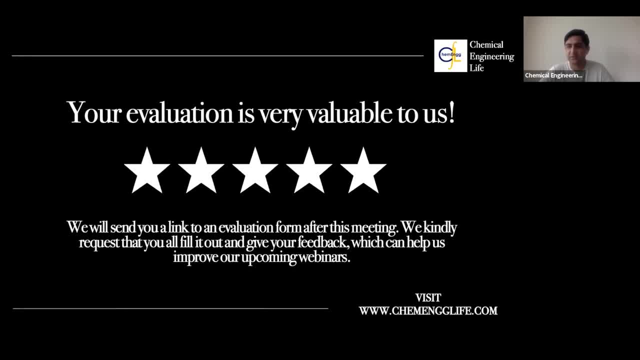 will be uploaded on our youtube channel as well, so you can also go there and watch it. if there's something you would like to say before we log off from mr lucretto, yes, so, um, normally i am open to any question. you have one of your technical.